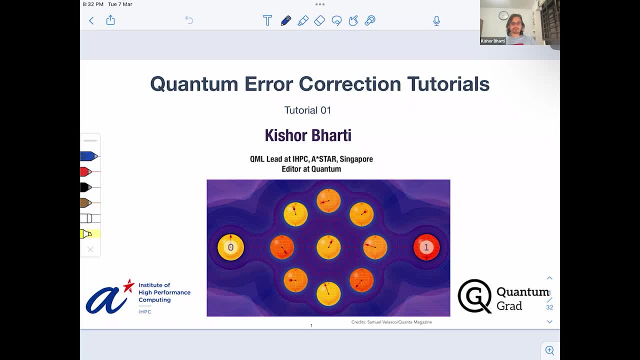 And it seems that there are around 60 plus people. So, yeah, like I hope I don't disappoint you. So basically, yeah, like I will talk about, you know, like quantum error correction, And so normally I like to, you know, like take questions in between. 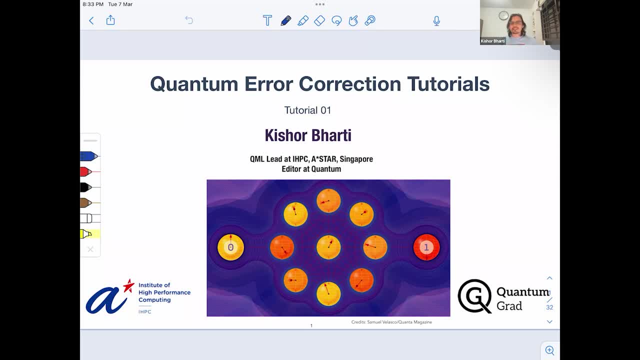 But here I need to you know like cover in six sessions all the content And I would like to take questions in between. Maybe you know like somebody can post that in the chat And I would prefer you know, like if other people, if they know the answer, you know like maybe they could respond. 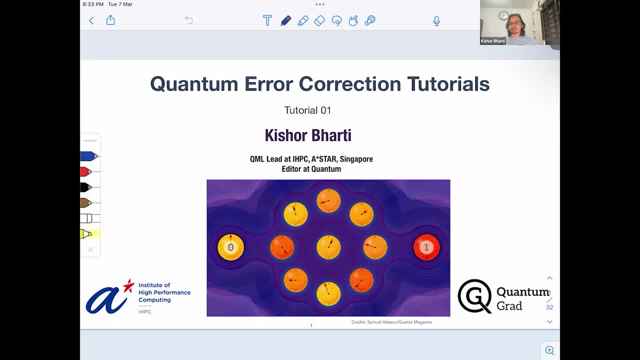 So in this way, you know like I may be able to like finish what I have decided, But yeah, I mean we could discuss more, you know, in the end So okay. so So, as you can see, like here: 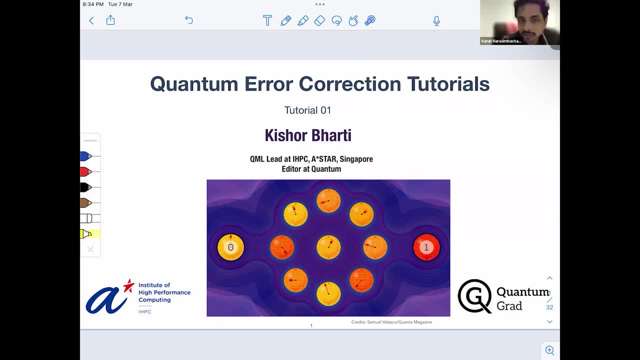 So so you can see, you know, like, do you plan to record this? Yeah, it's been recorded, Okay, Yeah, So, so, yeah, I mean. so currently I am at a start like, which is: 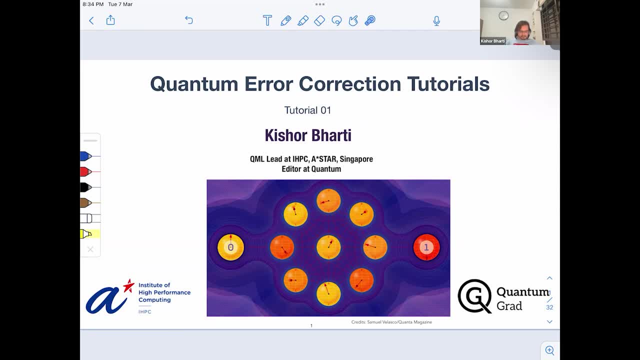 National Lab in Singapore And so I work at IHBC there And, yeah, like primarily my research interests have been, like you know, quantum machine learning device certification. Yeah, but recently, like you know, we moved into like error correction. 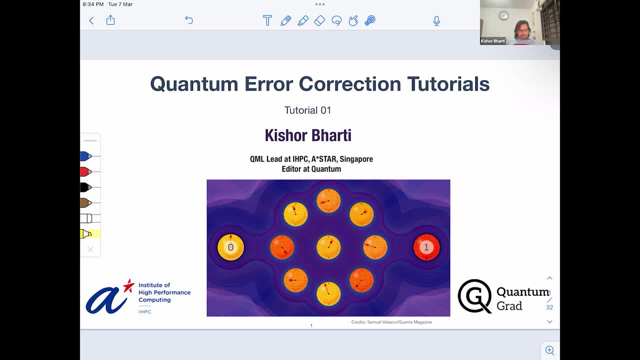 And so, like this, like you know, a series of tutorials. they will be later, you know, like posted on QuantumGrad, So like I mean also on QuantumGrad, So it's like I will explain, like, what QuantumGrad is. 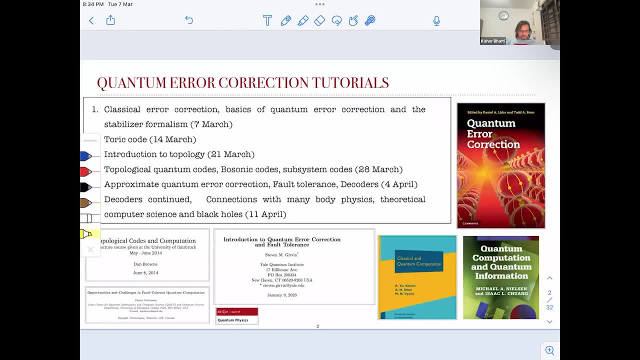 Yeah, So, so these are. this is the schedule. Like I mean you know, like this, this series of you know, like the six tutorials, And I think many of you already know the content, And, like you know, when it comes to like references, I mean I will follow mostly, like you know. 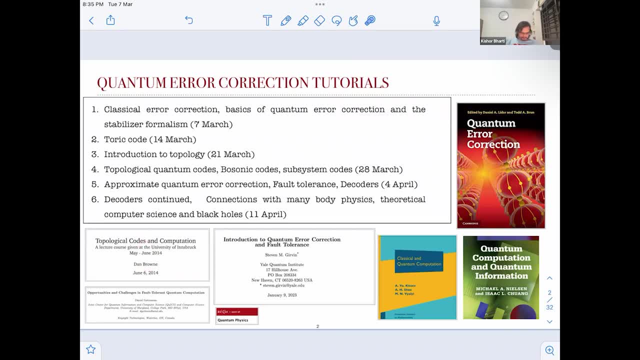 Dan Brown notes here, And also, you know, like, some of the chapters from this book on quantum error correction. Here, like I mean, sometimes I also, like you know, for some of the parts I will also, you know like, use papers from archive. 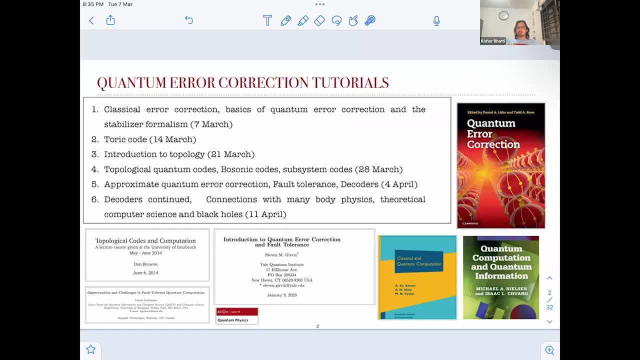 So I mean there are many papers so it's not possible to list. also, you know, like I mean, you can basically search them And, like you know, when it's required I will. you know, I will make a reference to them. 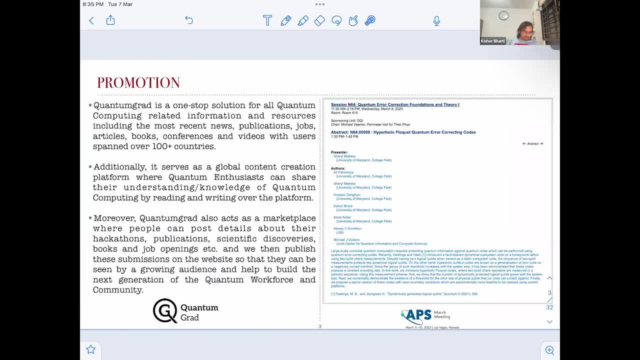 Nice. So there is a bit of promotion here. One thing about this: QuantumGrad. So QuantumGrad, you know, like I recently came to know about it, So like basically, yeah, So Sanjay from Sanjay Vishwakarma, from IBM Quantum. 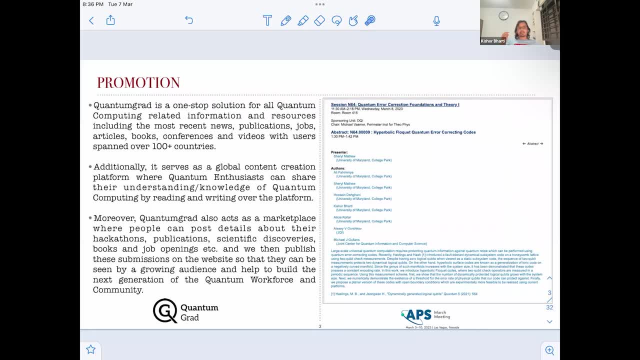 He, basically he and others, you know like they're involved in this. nice, I would say They call it one-stop solution. Basically, it's an open source platform where you know, like the content related to you know like quantum computing, is present. 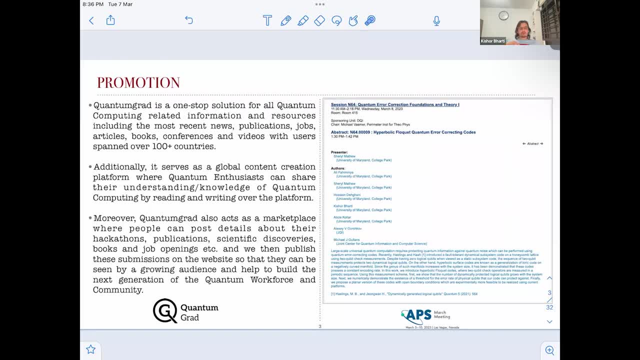 And yeah, I mean it's, I think, open source and everybody can access and all. And these are, like you know, tutorials. They will be later also hosted at QuantumGrad, So, if you want to, you know like, yeah, like more, get more information and all. 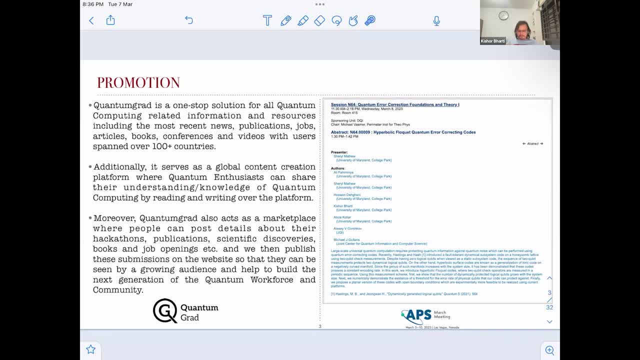 Maybe you know like I think it's a good idea to maybe subscribe On the side. you know like. I would like to just mention that if you are attending APS Mars meeting, there is this work where I'm involved, So you can see me here with my old affiliation. 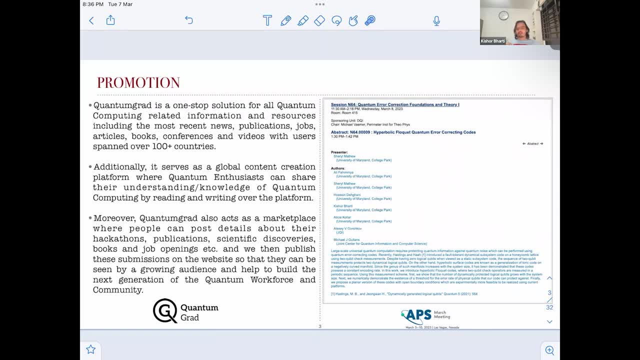 And it's on hyperbolic locate quantum error correcting codes, Like so it's like you know, like basically my friends and colleagues in Maryland And yeah, Like if you are in Currently, if you're attending APS, then please feel free to you know like you might like it. 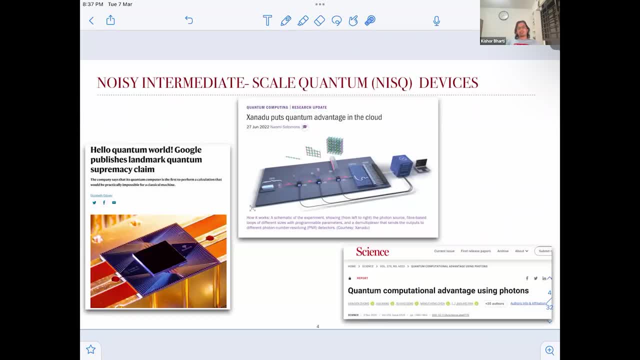 Okay, So we all know that you know, like the current era is basically, you know, like the NIST era, And it's called like a noisy intermediate scale quantum era. Like you know, expand it And there have already been, like you know, three. 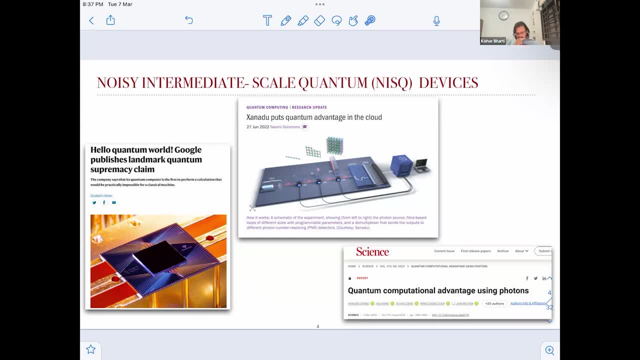 Actually four experiments And like, yeah, two experiments from USTC group And, like you know, but so far, like you know, yeah, like, first of all, like you know, how powerful these experiments were, like you know in terms of, like you know, classical simulability. 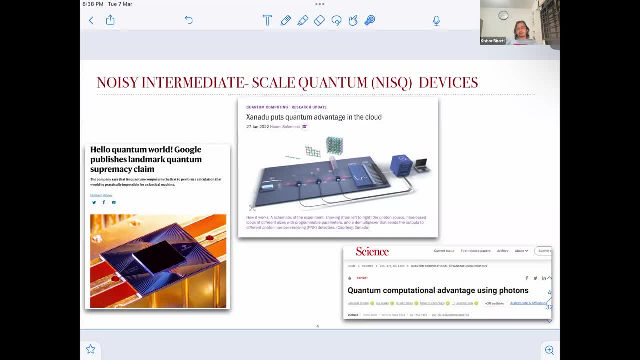 That's still debatable. And then, on top of that, the practical utility of these experiments Is, I would say, contested. I saw one paper, like you know, just three days back by Sheehan and Scott Aronson. 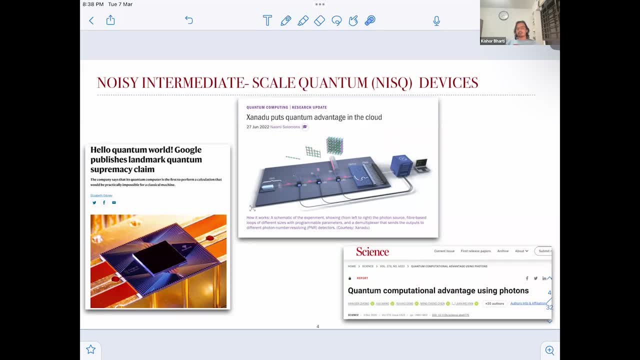 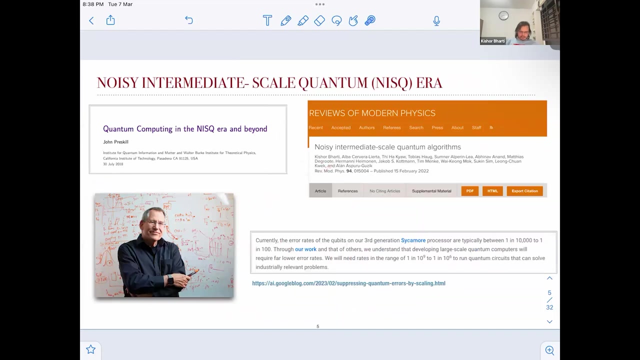 But I mean so far, the consensus is that you know, like, with the NIST devices we do not know any practical application yet. So you can see that You know like there is a review which I would just mention here. 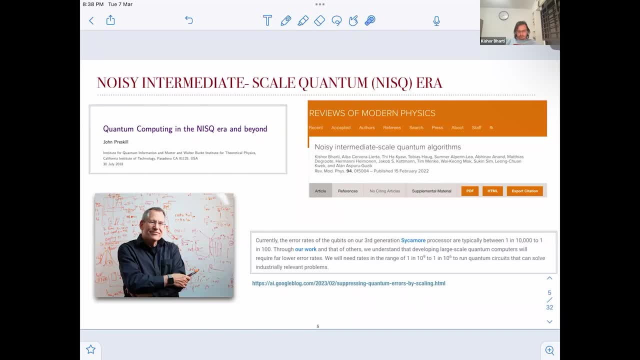 And the word NIST you know like, which was proposed by John Preskill, And you know like, basically, there have been a lot of work And you know like, you can see our review with. you know, like some of the friends and colleagues, 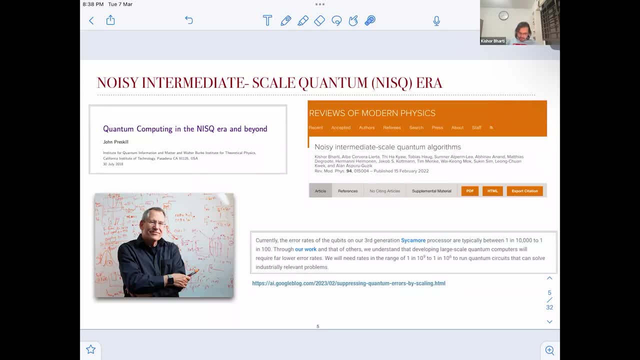 Yeah, And you can see, like you know, here I have put this recent, you know like, this paragraph from this recent experiment by Google Where they say that currently, you know like, in this recent experiment by on the Sycamore project, 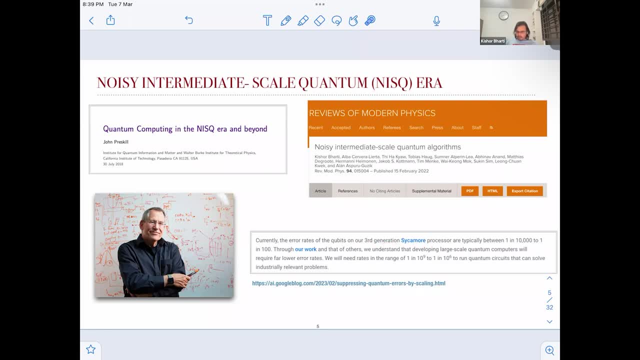 The errors you know like are between 1 in 10,000 to 1 in 100. And we will need rates in the range of 1 in 10 to the power, 9 to this much, to run quantum circuit that can solve industrially relevant problems. 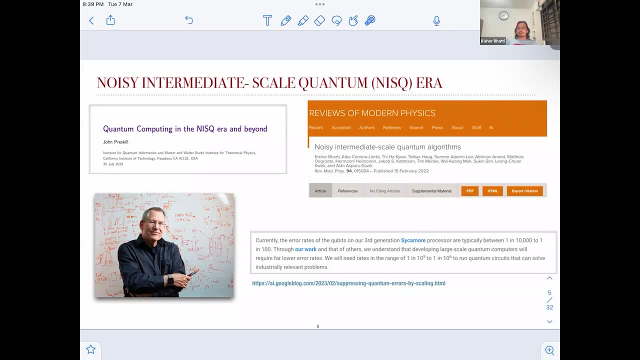 So I mean to reach there. I think it will be important to you know like perform quantum error correction And maybe you know like to Yeah, Like you know for noise separation. I think it will be, it will be quite important. 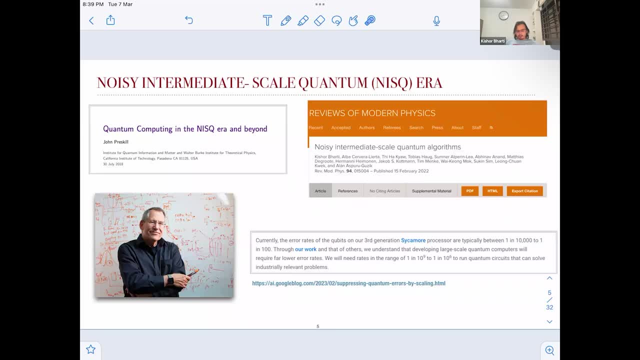 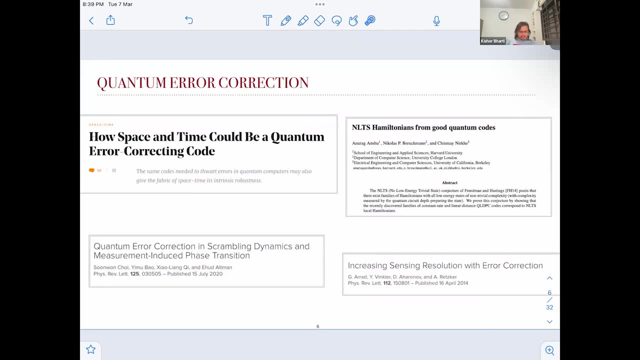 So, like I mean, so it very much elucidates, you know, like, the importance of quantum error correction for the community, And then on top of that, you know, like there are many other motivations also. So you know like, yeah, like it has relations with. you know like, yeah, like, general theory of relativity. 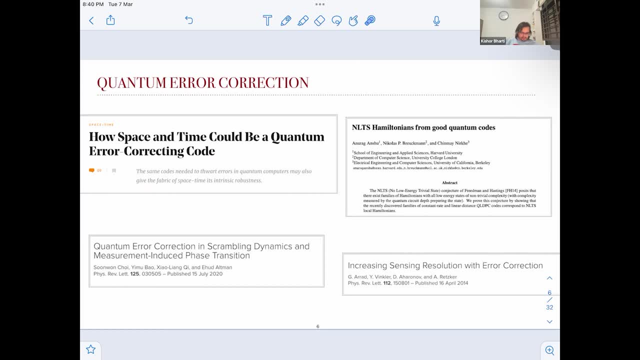 I mean basically black hole theory, Yeah, And also you know, you know like physical physics And then, like you know, many body physics. Then there was recently, like you know, a breakthrough in theoretical computers science which used, you know like a kind of like you know like error-correcting codes called quantum LDPC codes. 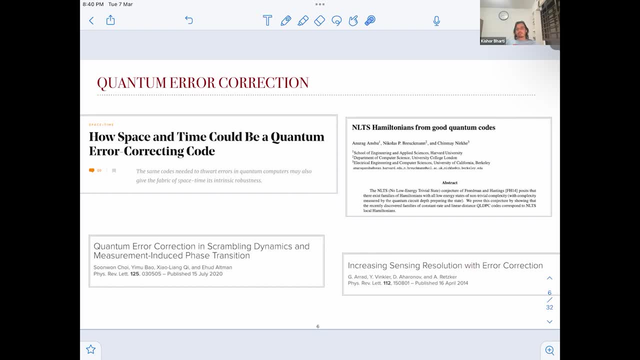 And then also in metrology, you know, like there are, you know there have been a series of papers which, have you know, looked at how quantum error correction can you know like, improve a phenomenon, uh, improve uh, metrology mice. so so there have been, like you know, a series of works and uh and 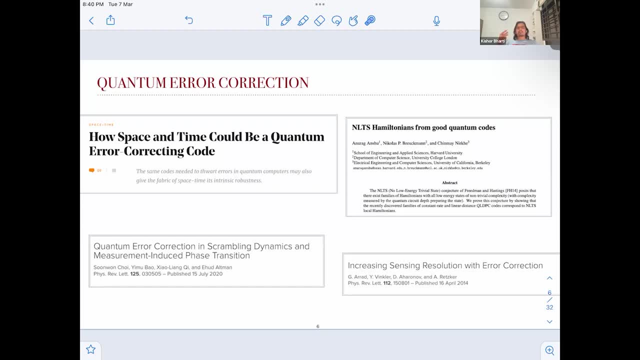 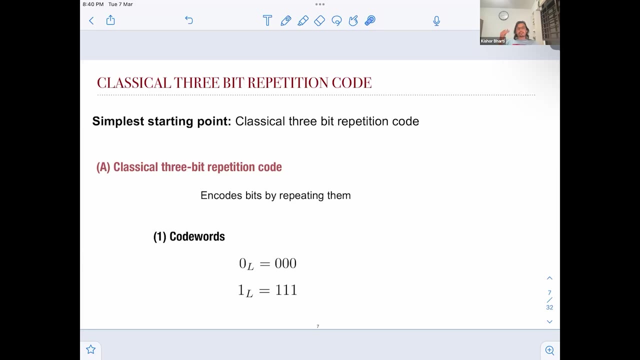 like i mean, yeah, like it makes sense that you know like we need to, we should understand quantum error correction. you know like, if we are interested in any of these topics, okay, so today i will, you know, like, focus on. basically there are three parts, like the first. 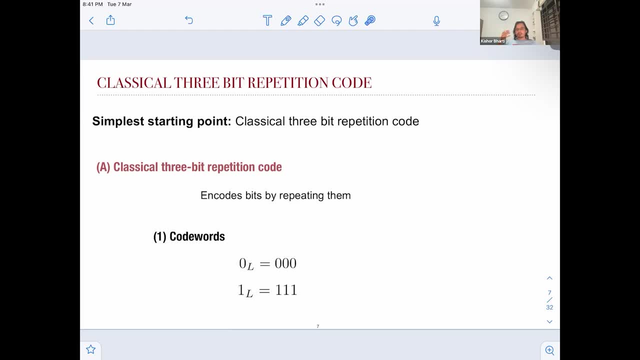 part will be the classical uh classical code, which will be a classical three-bit repetition code, and then i will move to a quantum three-bit repetition code and finally, i will talk about stabilizer formalism and show you that how you can understand the quantum three-bit repetition code. 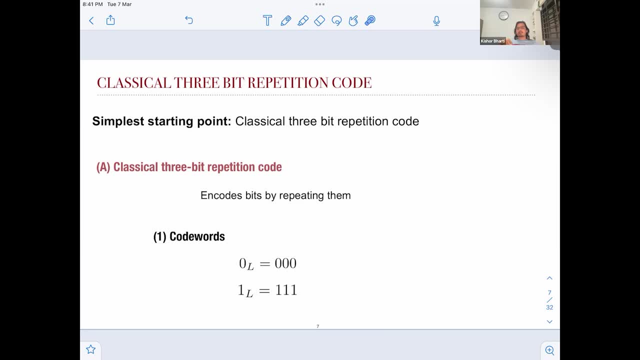 in the stabilizer formalism. so this part i could you know like many of you might find it elementary, but uh, like in the later tutorials, when we talk about tori code, others, you know like it will build on, like you know. so, yeah, like i mean, um, i apologize if some. 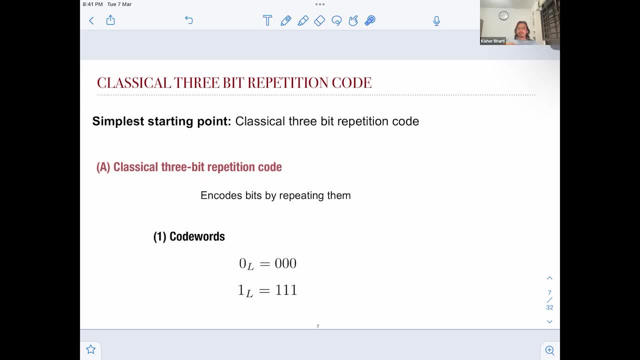 of the content here. you know like is uh like it may look elementary, but i i think uh it will give uh gradually. you know like pick some case, so let's look at. you know, the simplest starting point when we think about, you know like, classical code is the classical three-bit repetition code. 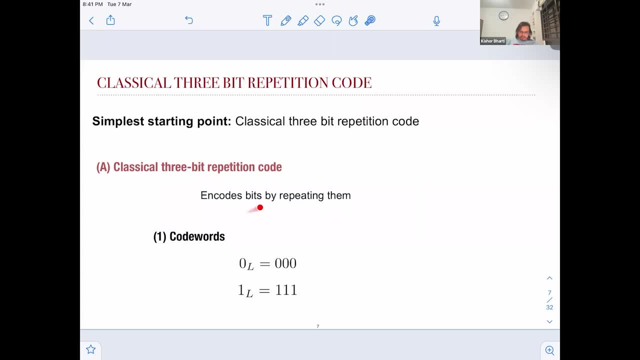 so what is this classical three-bit repetition code? it basically encodes bits by repeating them. okay, and three bit basically means that it repeats it three times. so you take zero and you know like and you write it three times and you know like you get this zero logical and if you repeat one, 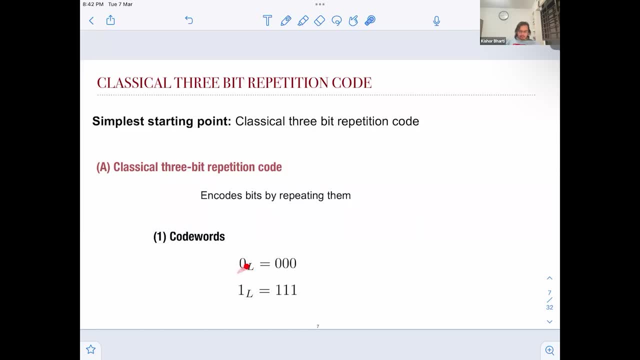 three times you get one logical. so you have the zero logical here and you have the one logical here. so so you know, these are the code words. now the error which can happen in classical code is a bit clip error. so your zero can become one, your one can become zero. 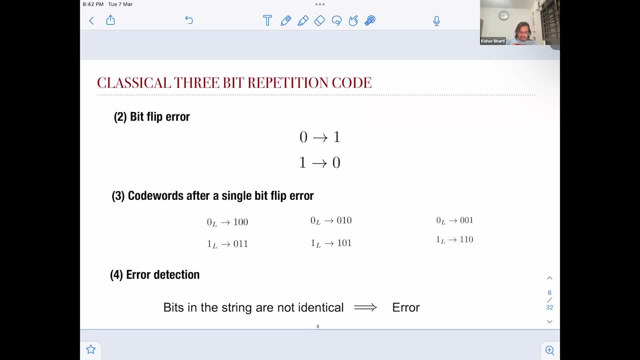 for example your zero logical. you know like, let's say, if the first belief bit clips, then it can become one zero, zero. if the yeah, like for for the one logical, it can become zero, one one. and similarly, let's say the last bit clips, zero logical can become zero, zero, one and one logical. 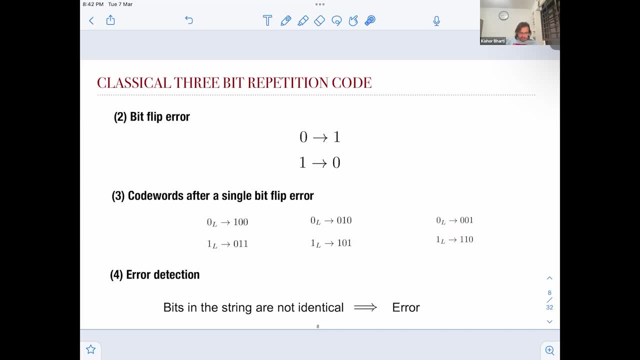 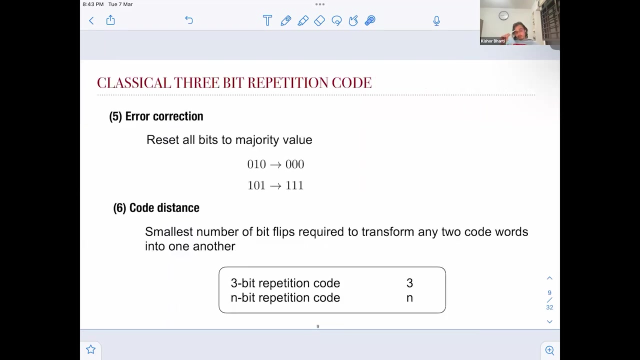 can become one one, zero. next, simple and error detection here, uh, is like also quite simple. basically, you look, you look at your- yeah, like core strings and if you see that the bits in the string are not identical, then it means some error has occurred. uh, so how do you correct? like, even like when you 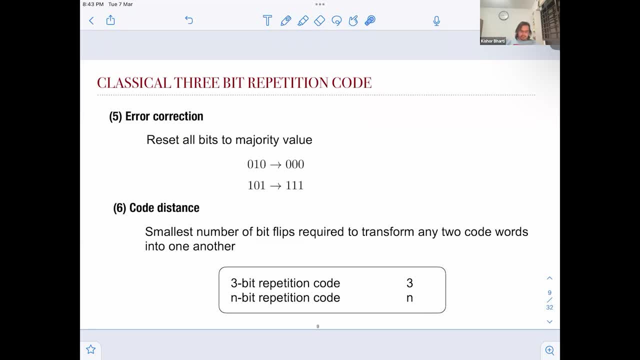 have detected an error. so that's also simple. basically, you reset all the bits to majority value. so, for example, if you have 0 1 0, you will you know like, write it at 0 0, 0. or if you let's, you will you know like you can, yeah, we will, uh, you will set it to zero, zero, zero. so basically, 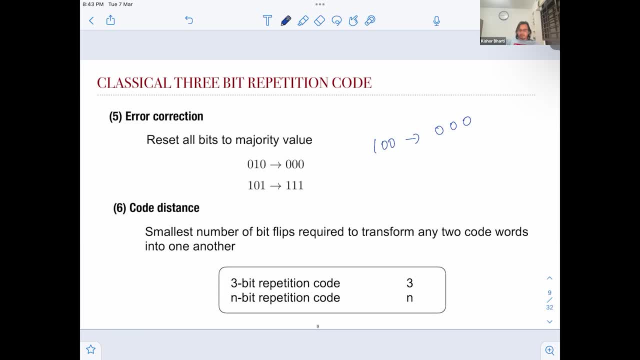 you will, like you know, reset all the bits to whatever the majority value is of the other side. and then the question becomes like what if you know, like let's say, that there are three, uh, three bit slips, so for example, let's say zero, zero, zero clips to. you know, like one, one, one can. 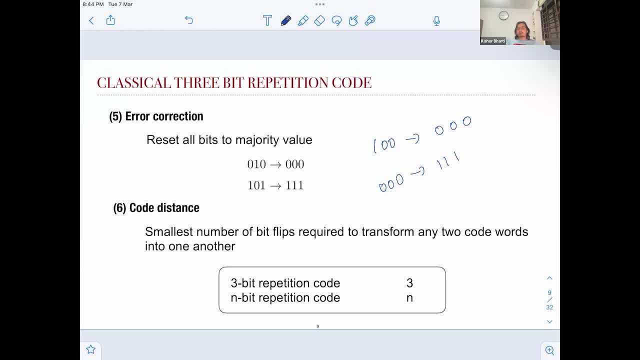 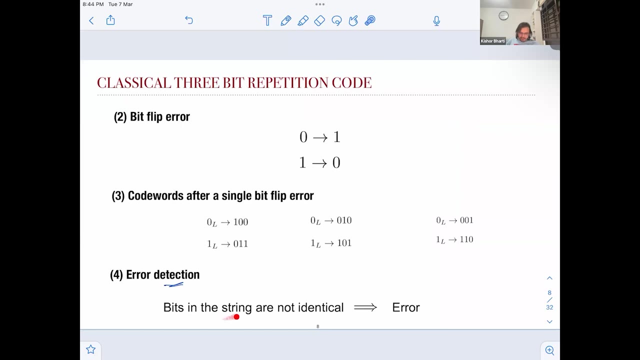 you still: uh, detect there. now, that is not possible to detect, right, because uh, here, like you know, i mean, as we, like you know, mentioned before, the way you detect the error by is by looking at whether the bits in the string are identical or not. and let's say, if all three bits flip, then you know. 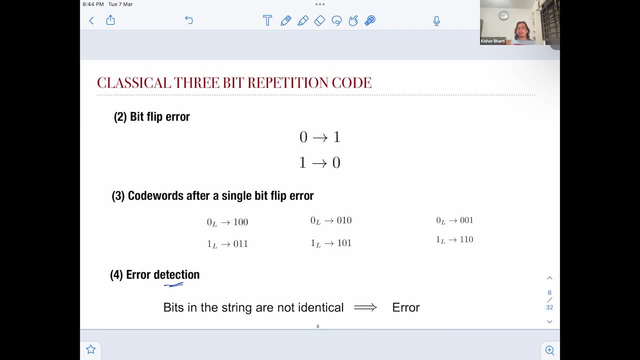 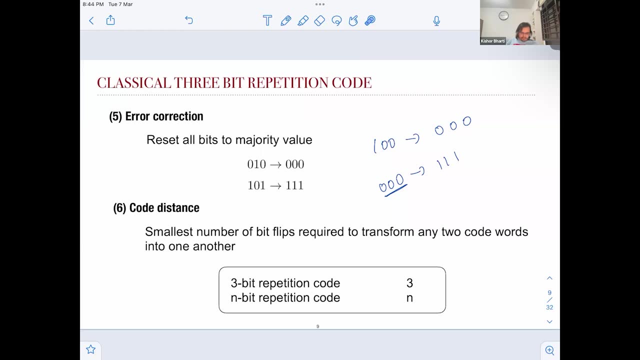 like the bits are or are all identical and you will not be able to be able to, you know, like, detect it, so. so code distance, you know, like uh captures. you know this notion of uh, like, uh, uh, whether you can uh detect the error or not. so code distance basically means the smallest number of bit. 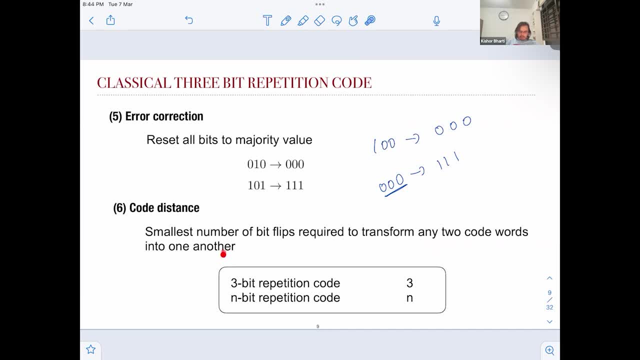 clips required to transform any two code words into one another. so you have, like, the two code words that we have are basically zero, zero, zero and one, one, one, and you need three bit clips to basically transform one code word into another. so for a three bit repetition code, 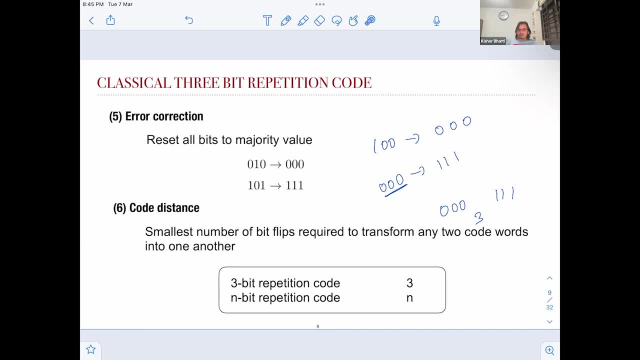 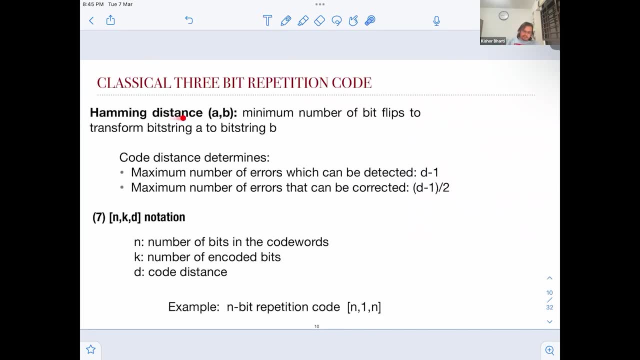 the, the distance is three. if you have a n bit repetition code, the distance will be n. so there is this notion called hamming distance which captures, you know, like the notion of uh distance for the classical code. so basically, let's say you have two bits in a and b. 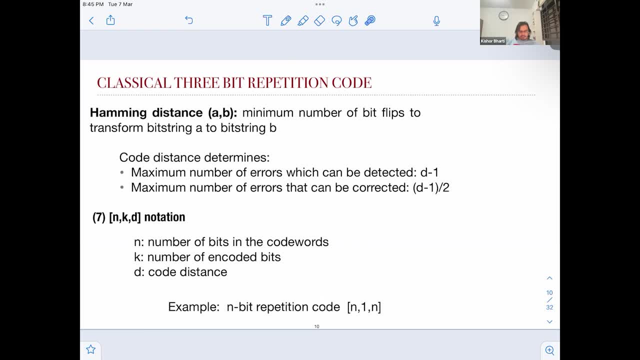 the minimum number of bit flips to transform bit string a to bit string b is called the hamming distance between a and b. so you can see that you know like, basically, if you have a bunch of uh- like you know- uh codes, uh, code words, uh, you need to calculate the minimum hamming distance, like you. 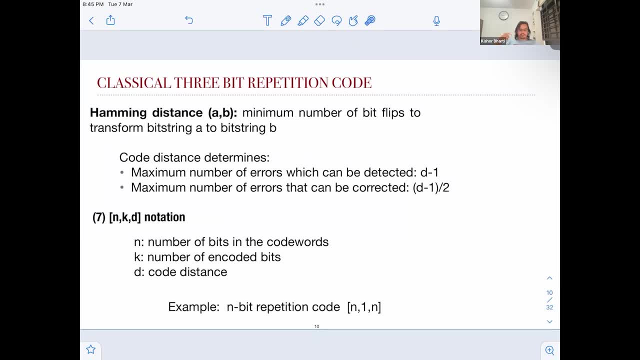 know among all pairs of, you know like code words and that will be your distance of the code. so, yeah, like everything, uh, so you can see that the maximum number of errors which can be detected is obviously one, because if it, if it's d, then the the error correct error detection scheme will not work. 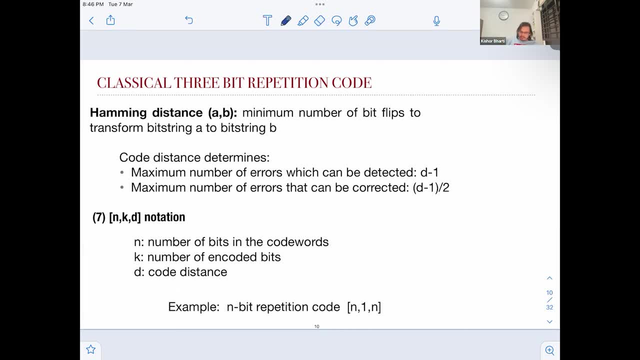 and the maximum number of errors that can be corrected. that will be, you know, like d minus one by two, yeah, and what? because, uh, uh, because otherwise your majority, uh, like you know, majority reset scheme will not work. so that's why you know, like uh, the number of error that can be corrected. 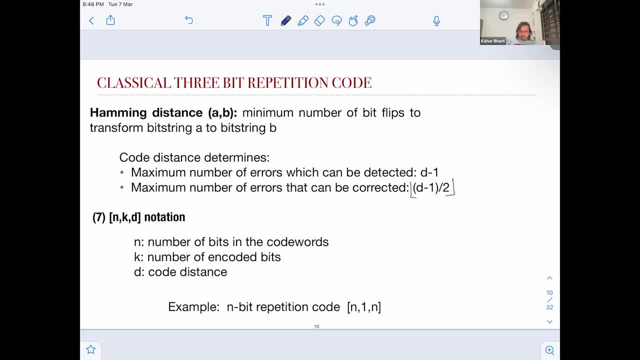 is, you know this, uh, this floor of d minus one by two and the, the number of bits, number of error that can be detected, you know, like is basically d minus one. so so far we, you know like, we talked about, like you know uh, errors, uh like code words, errors, uh, yeah, like, just like replacing you like. 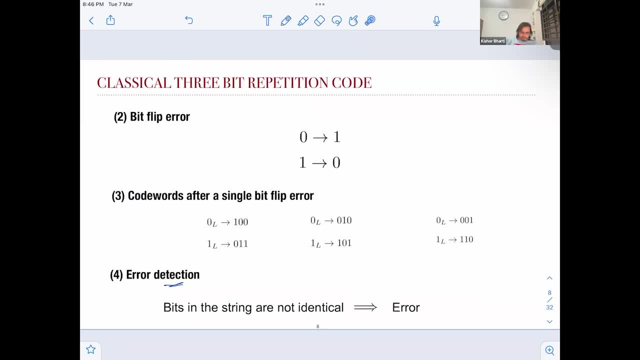 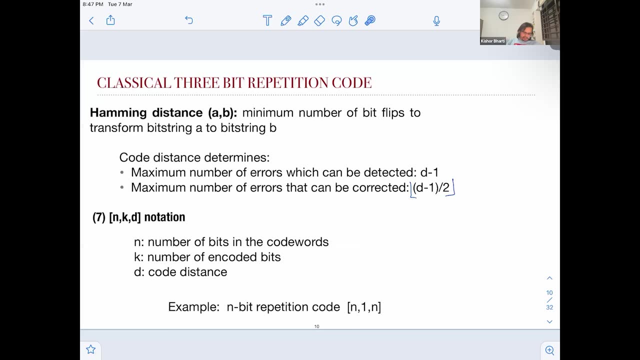 so code words and then errors, and then, uh, what happens to code words after the error, error detection, correction distance. now you have, you know like, let's say you have uh, n number of bits in your code words, like, and let's say k is you know like the number of encoded bits. so in other cases, let's say the three-bit repetition code, we are. 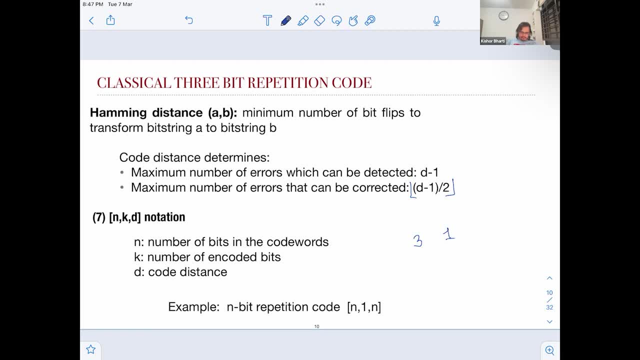 using three bits. to you know, like in code, one bit and let's say d is the. you know like the code distance. so in our case you know, like for the three-bit repetition code, the distance is three. so for such cases, you know like you, you write it as there is this mutation in classical error. 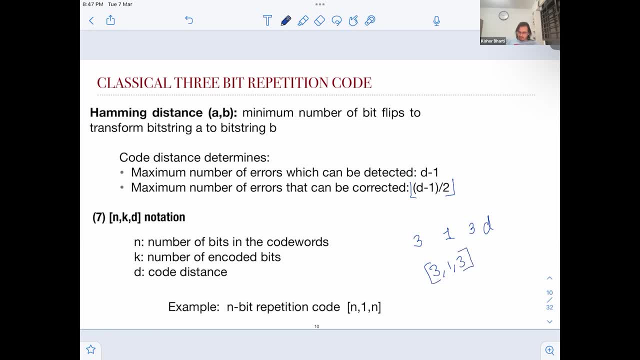 correction, which you know rightly, like three, one, three, basically. so so this is your n, k and d and let's say instead: if you are interested in like n bit repetition code, uh, it will become n, one one, n, one, n. so you are using basically n like n bits to encode one bit, and your distance is n. yeah, 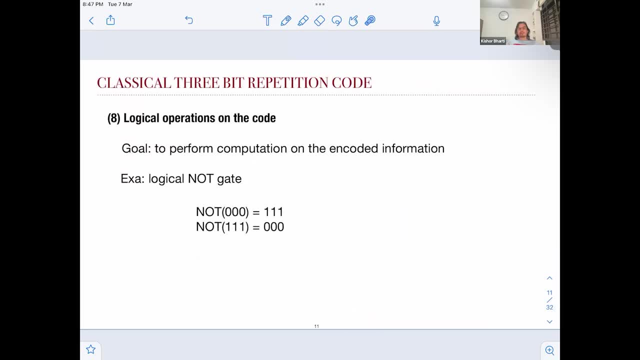 so so what are the logical operations on your uh photo, like uh, let's say the here the goal is to like perform the computation on the encoder information like you would. you would like to perform some computation like you have encoded. but i mean, there is you, just. 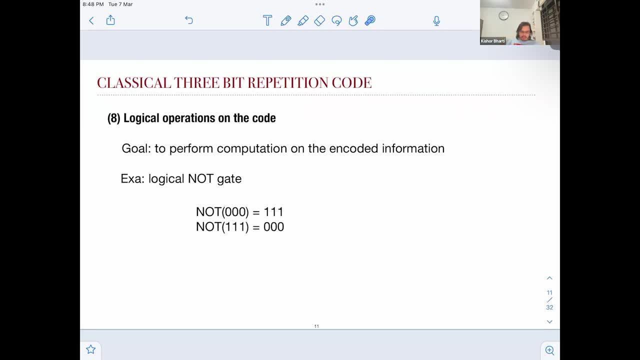 do not want to store it. i mean, like you would like to perform some computation and one of the computation you know like is like they are applying the not built, so the. so the action will be same, as you know, like what you have in the unencoded case, so the, for example, if you 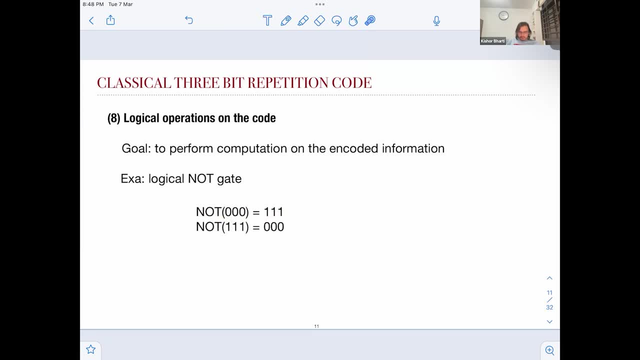 apply the logical not to get on zero, zero, zero, it should send it to one one one. and when you apply to one one one, it should, you know like, send it to zero, zero, zero. so you see that your logical operation they keep your. you know like, uh, uh, like they keep your code words, like you know. 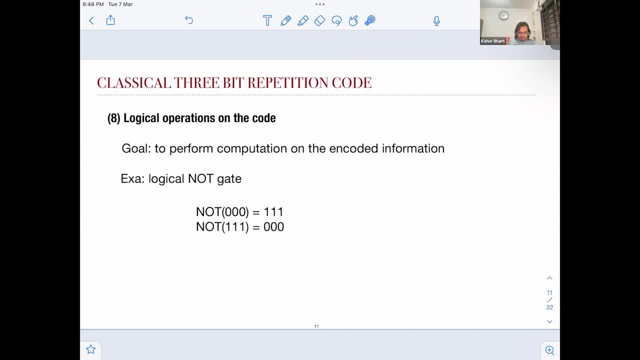 they map one code word to another. you know like yeah, okay, like here least, yeah, so. so then i mean later i will talk about this notion of code space and i will tell you that this logical operation, basically you know like uh, uh, keep your the quant. you know. 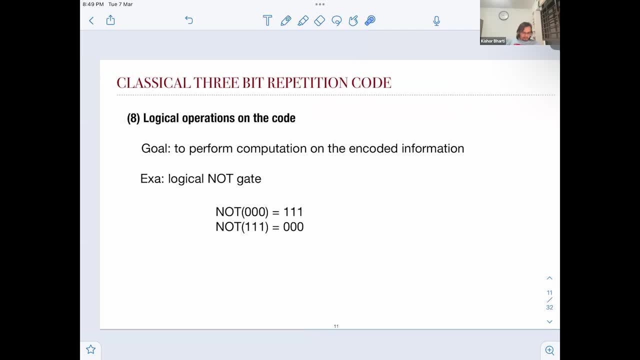 like the state within the code space. yeah, so i mean so for the moment. you know like we just discussed the classical uh three bit, or you could say you know like n-bit repetition kit, that is repetition code where we talked about. you know, like the encoding, the error, yeah, like, and the. 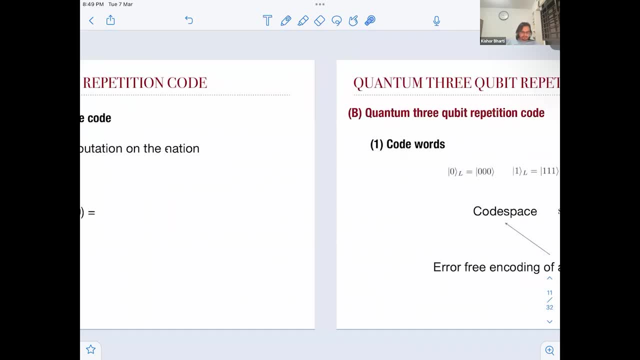 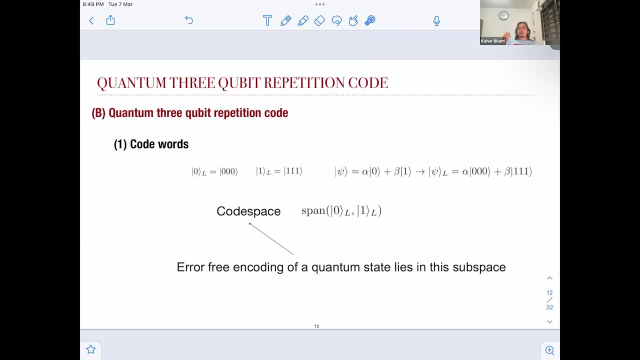 distance, nkd notation, the logical operations and so on, so so. so this completes the classical part. let's look at the quantum part now. so now we look at, you know, the quantum three-bit uh repetition code. so here, like you know, similar to the classical case, we have your zero logical will be, you know, like zero, zero, zero. the one logical will be one. 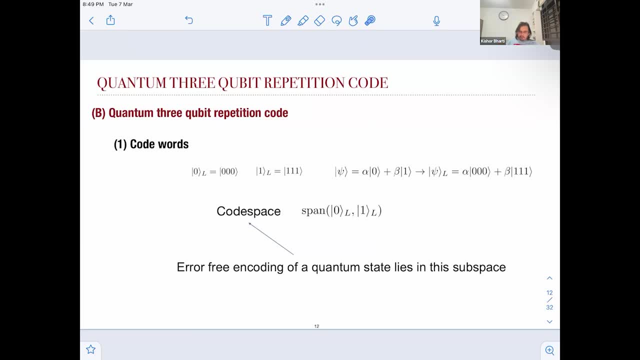 one one. yeah, like basically you repeat it. and so, which means that you know, like, let's say, you have some quantum state, alpha 0 plus beta 1, you will encode it as alpha 0, 0, 0 plus beta 1, 1, 1.. so you can see. 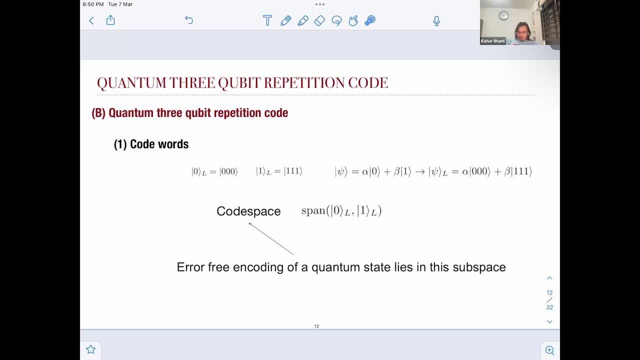 that, like the here you know, like this, all possible you know, like, like psi that you have here belongs to the span of zero logical and one logical you know like, which we have defined here. so this is your code: space and basically error free encoding of a quantum state. 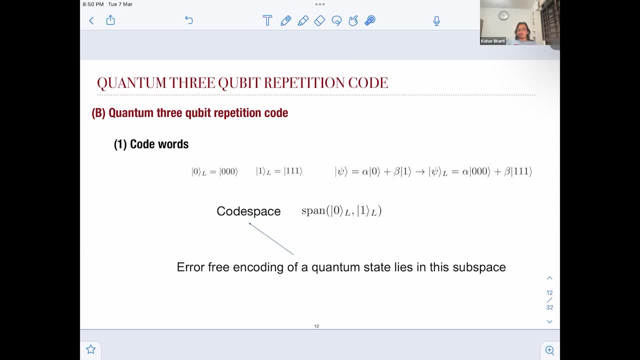 lies in this subspace. yeah, so i think uh, this makes sense. so that's how you know, similar to the classical case, we have defined the uh code word for the quantum case. now let's look at the errors. so here you can have, you know, like bit flip error. 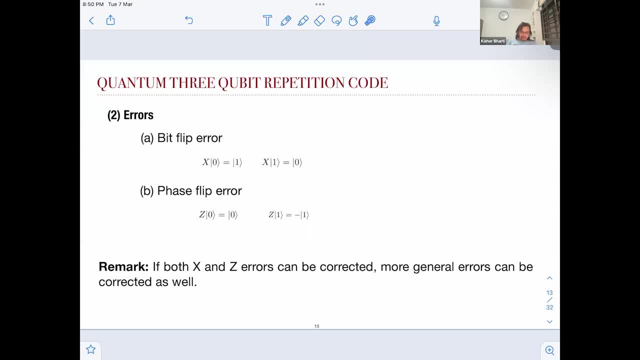 or a phase flip error. so a bit flip error. basically, you know like a, know that it takes your x, like. when like is divided by x, like takes your 0 to 1 and 1 to 0. so you know that it's given by this matrix. you know like 0, 1, 1, 0 and when you act it on, 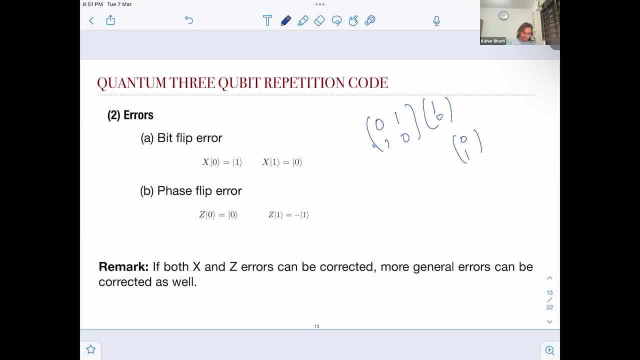 1, 0, it will give you 0, 1 and when you act it on 0, 1, it gives you 1, 0 and the phase flip error. basically, you know like it is, it's just uh. you know it just uh adds: uh, you know sorry. 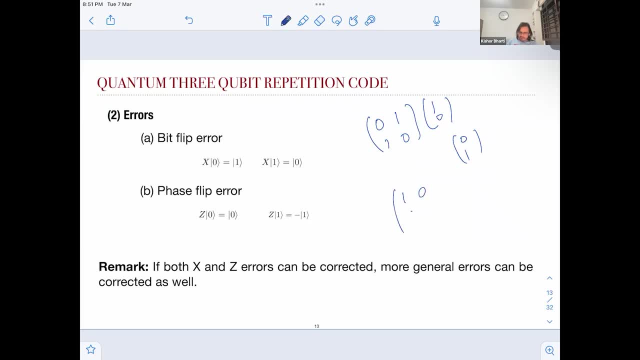 so it'll just add some phase in front of you know, like one. yeah, so if both x and z error can be corrected, uh, more general errors can be corrected as well. so this you can think what you know like: uh, basically, even though you know the quantum errors can be continuous. 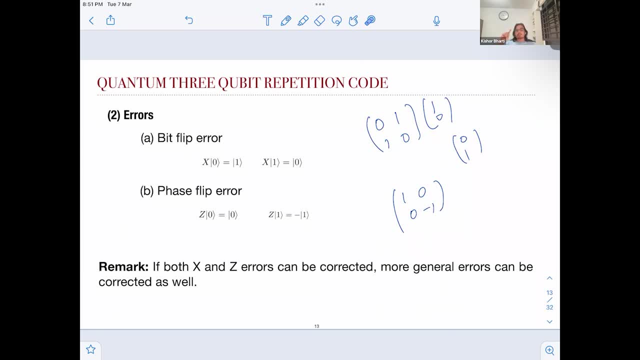 you know like by, by, just by, you know like, looking at your x and z error, you can, uh, you know like, so basically it's a way to discrete. a lot of your result as well is quantum errors and uh, and you can, you know like, correct more general errors as well. 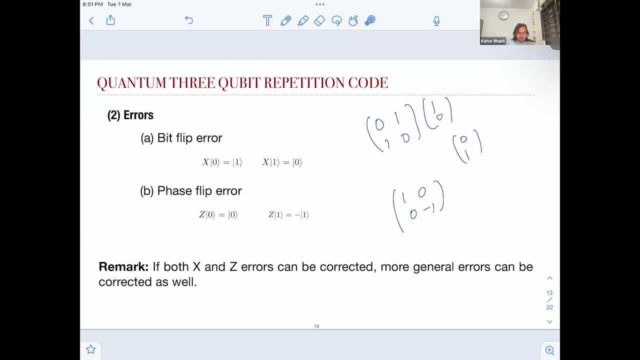 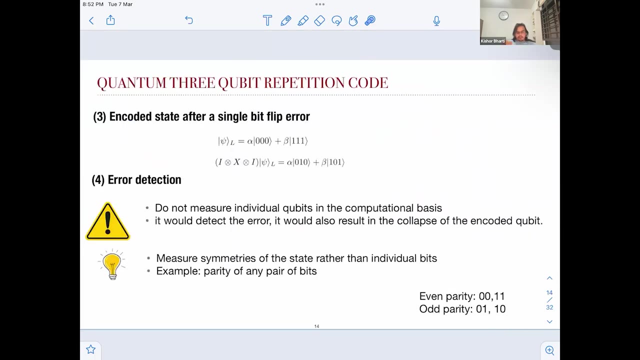 so, uh, so we talked about errors. so like i mean, so you know. so, unlike the previous case, we we not only have- we don't only have, like you know, bit clip error, but we also have this phase. nice now, what happened to the encoded state after a single bit clipper, for example? so, 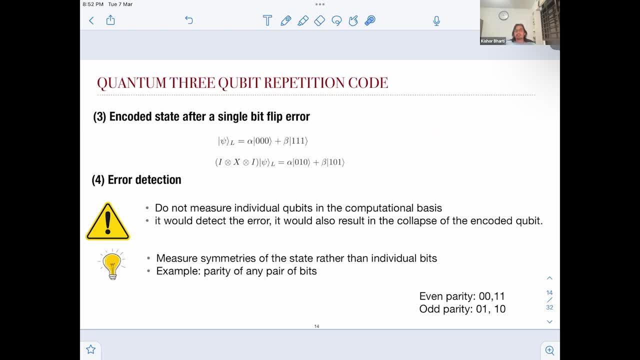 since we are looking at, you know, repetition code, we will. you know like we will be interested in, like bit flip error. so so let's your. the logical state that we had was alpha, zero, zero, zero, plus beta, one, one, one. now let's say, you know like you act. let's say the second bit, you know like, uh. 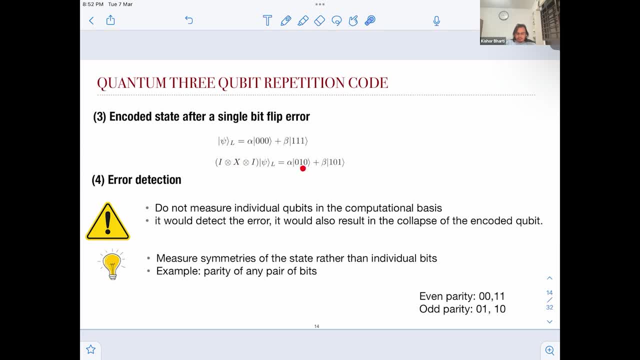 the bit flip. error happens on the second qubit, so it will just, you know like, flip your second qubit so you get zero, one zero plus beta one, zero one. so now the again the same question comes: okay, like some error has occurred, and can you detect it? now, in quantum case, you know the the situation is a bit tricky because 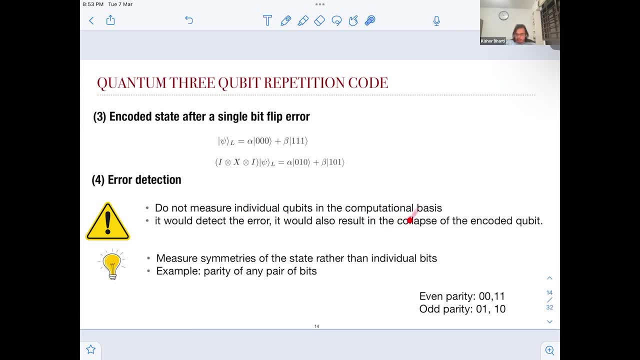 you should not, i mean. i mean, if you try to measure the individual qubits in the computational basis, you will detect the error, but it will result in the collapse of the encoded qubit. so we don't want that. i mean we want to, uh, protect the information, right? so the idea is: 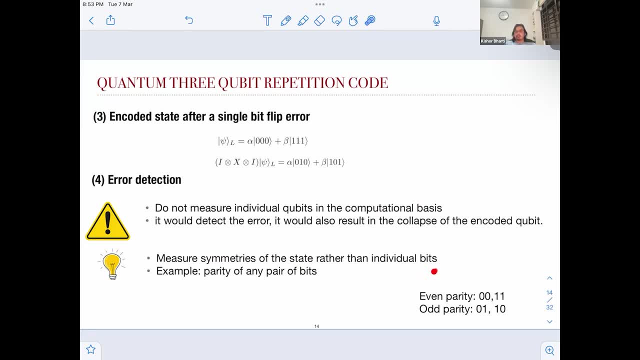 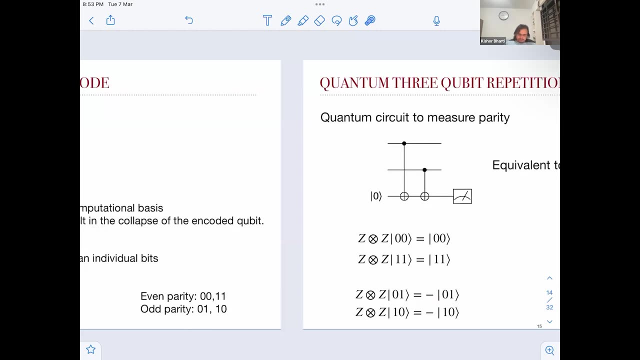 that you measure symmetries of the state rather than individual bits and uh, one example could be, you know like, a parity of any pair of bits. so the event parity, you know like something like zero, zero, one one odd pi pi. you know like zero one one zero. so let's look at, you know like, how it works. so 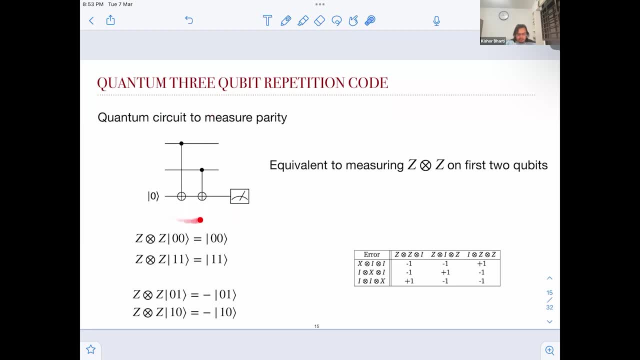 for example, you know, like uh, so this is a circuit which can be used to, let's say, if you have any two qubit, this can be used to measure the parity and this can be, you know, like shown to be as equivalent to measuring jet tensor j. on the first you can work out the details, but let's look at, you know, 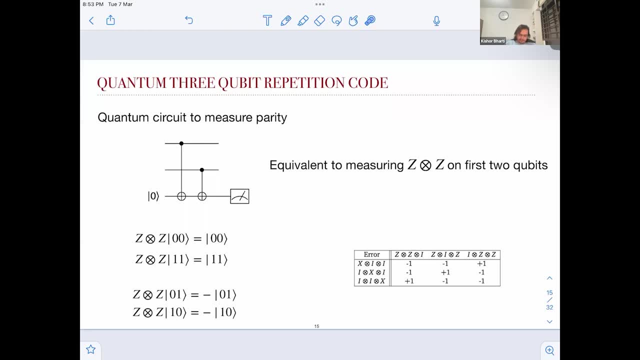 like all this jet tensor, jet capture, you know like what we are interested in. so when you act, when you look at, you know like zero, zero, the parity of zero, zero is uh uh zero. and jet tensor j, when it acts on it, you know like it gives you, you know like you get plus one right and then jet. 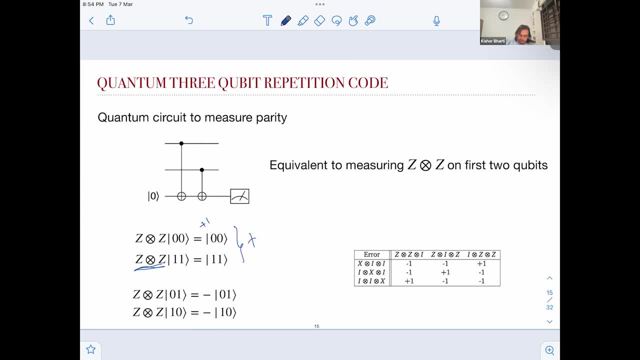 tensor j on one one that's, that's also basically belong to the plus one, uh, like you know, subspace. on the other hand, zero one and one zero, their parity is one and this belongs to, you know, like the minus one subspace. so you see that, uh, this jet tensor j, basically it captures. 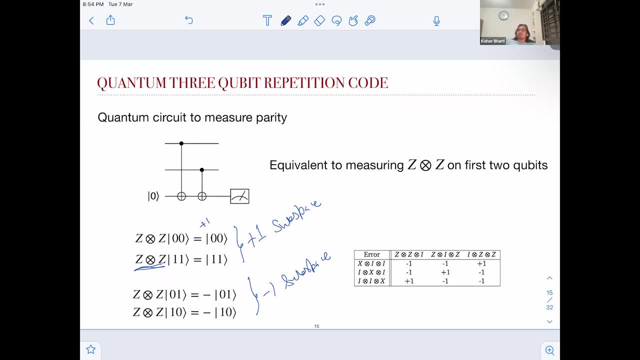 like you know it, uh, it captures the parity of the of the pair of qubits you know like, on which it acts. so so here i have, you know, like this, i added this table which you know like, looks at a, you know suppose, the first bit. like you know, the error happens on the first bit and when you act by you, 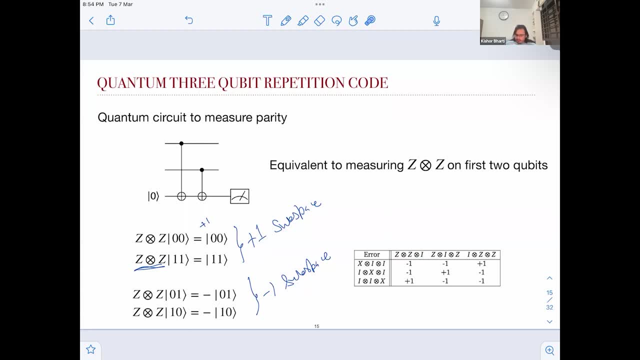 know like jet tensor, jet tensor i, you will get a minus one. you know like so, because you know the parity of the first and second bit. you know like that will not be same. so that's that's why you have a minus one here and and this one also will give you minus one. but you know like, because these 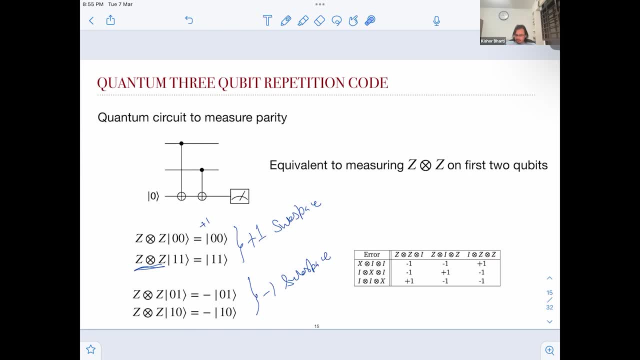 two bits are not top. i mean your this jet tensor jet. you know like, uh, like, here no error has occurred, you will get plus one. you know the jet tensor jet will not give you anyway. now it's crucial to see that, as whenever your error, like you know, anti commutes with the, with the operator, you know that. 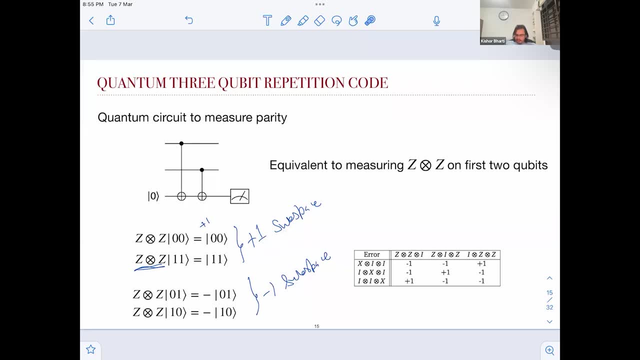 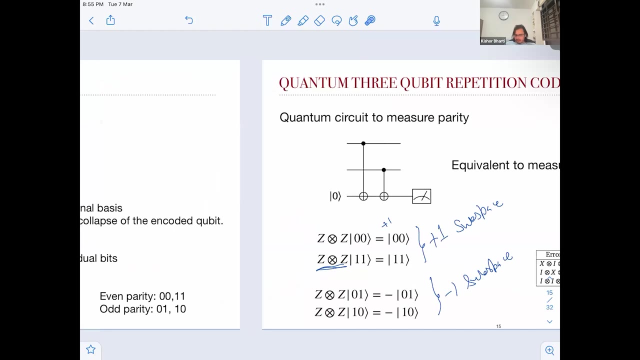 you are measuring, you get minus one. on the other hand, when it commutes with the operator that you are measuring, it will give you plus one. nice, so so, so, this is the idea you know, like you. basically, you measure certain uh, you know, uh, like symmetry, like you know here, the parity and and the object that you measure for 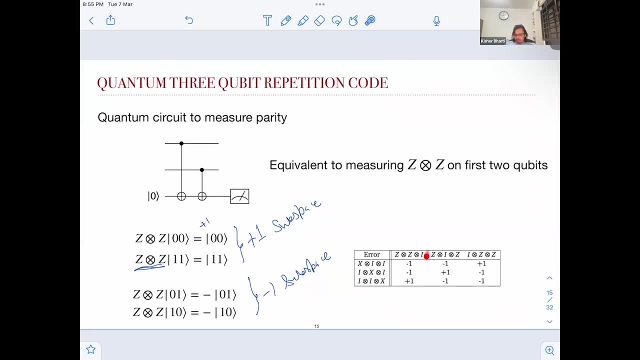 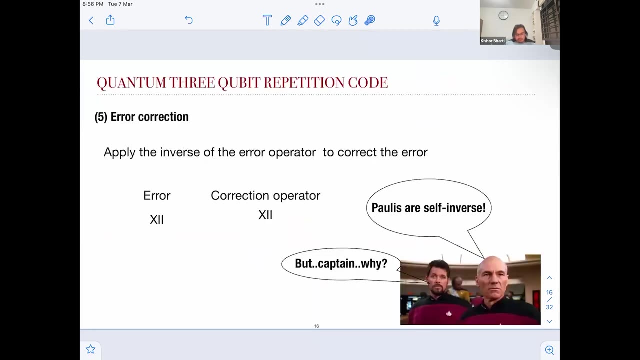 example, for the uh three qubit repetition code is basically jet tensor z i, then z i z and i j z, and that, should you know, like help you to detect the uh detector. nice, so finally you know like it becomes like: how do you correct the errors? so, to correct the error, basically we apply the inverse. 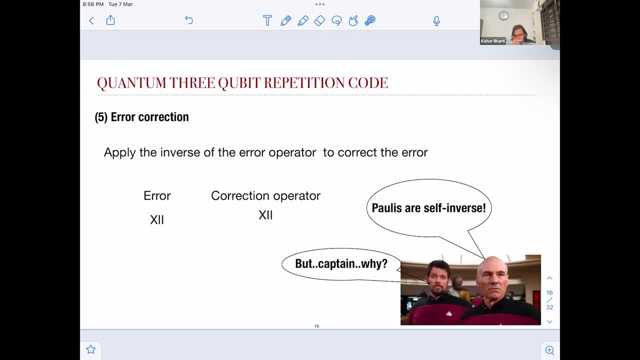 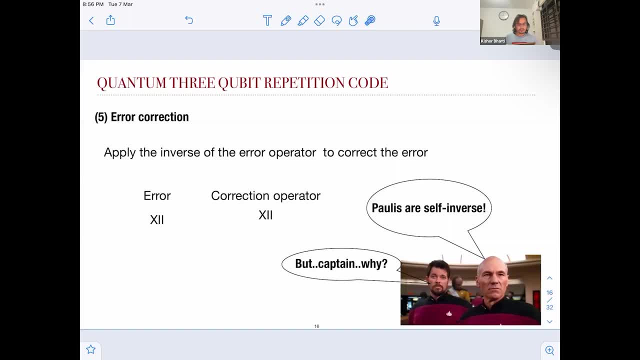 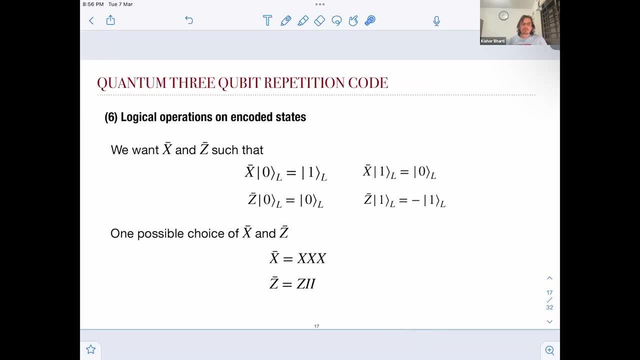 so because of that, you know, yeah, error correction is quite uh easy in this case, okay. so finally, i mean okay, we come to this notion of you know what are the logical operations on encoded states. so we want basically, uh, you know the logical operations x bar and z bar, such that you know like, uh, similar to like. 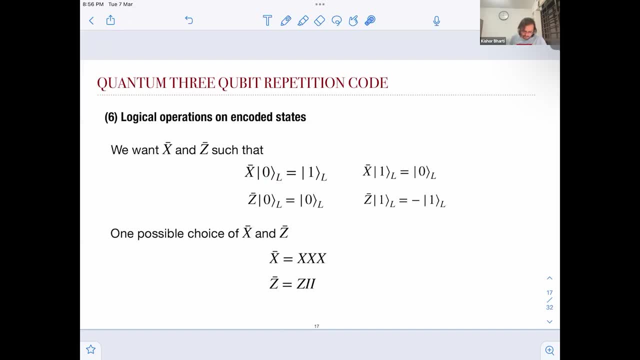 regular x. when x bar acts on 0 logical, it gives you one logical, and then it acts on one logical, it gives you zero logical. similarly, zedwar, when it gives you works, acts on zero logical. it gives a zero logical but picks up a face in the case of one logical. 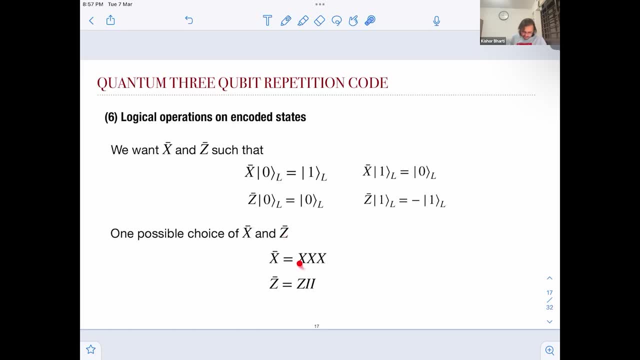 so one possible choice of x, y and z bar that you could have is basically x, x, x and zii. why that is the case? like you could see that when you have xxx and you act on zero, zero, zero, it will become one, one one. and similarly, if you act it on one one one, it will become zero, zero. 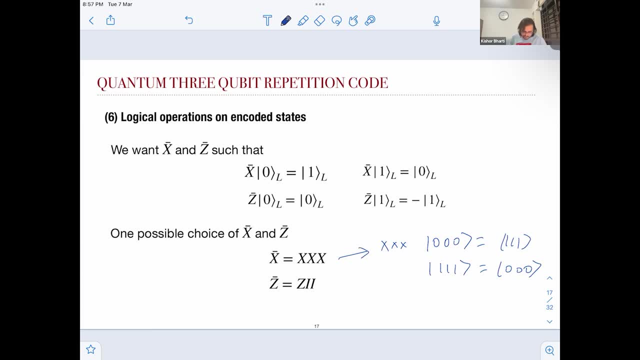 zero. so you see that this, this acts as a nice choice of you know like, uh, uh, logical x, like it satisfies the condition that we require. similarly, like you know, code z: yeah, maybe, like you know, here you could just select zii. and you see that you know, like, when you act it. 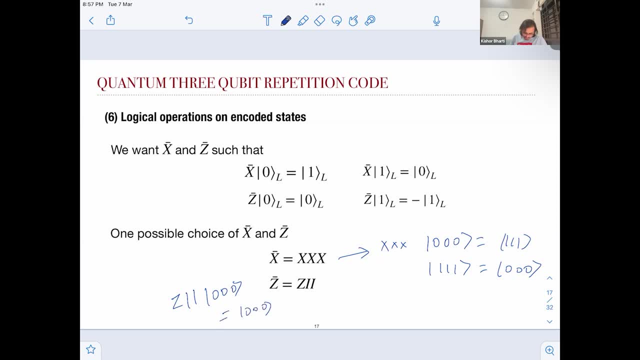 on zero, zero, zero. you know like it will give you zero, zero, zero. but when you act it on, you know like when you act it on zii on one, one one, it will give you minus one one, because you know like you have z on one of the like qubits, yeah. so you see that. 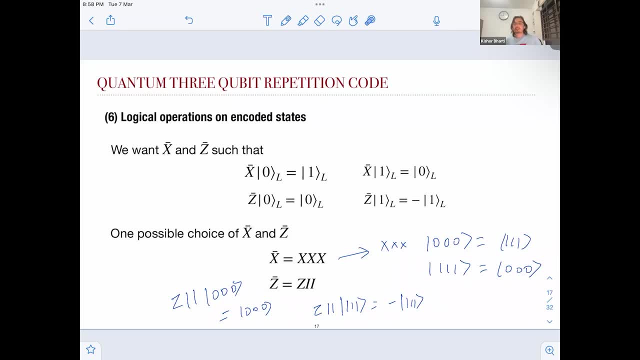 this is a, this can act, as you know, like, as a. so at the moment we are just- uh, we are not systematic, like just based on intuition. we are building, you know like, what will be the logical operators. how will you, you know like, detect the error? but later you will find all this process can be automated. 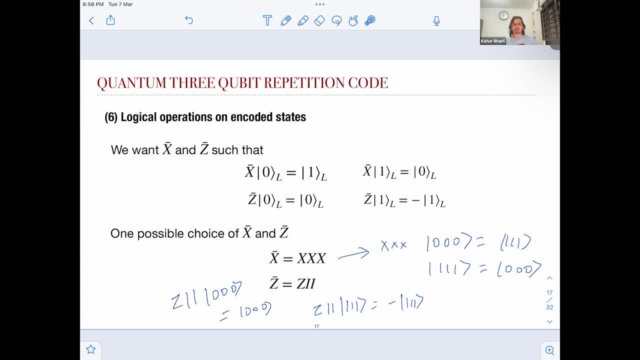 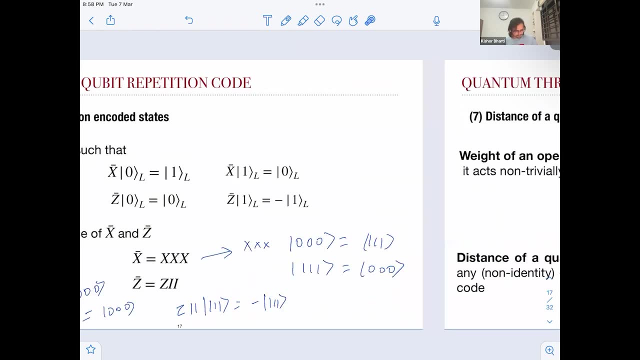 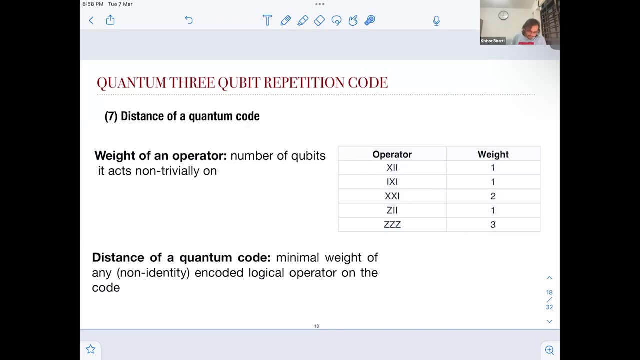 like using a simple idea, pro group theory, you can, uh, you can. just, you know, like, uh, look at the problem of the problem, so by using this method, you will be able to've, you know. look at the con artist, so here I am showing you how, uh you can deduct z to your operator. we can also look at the 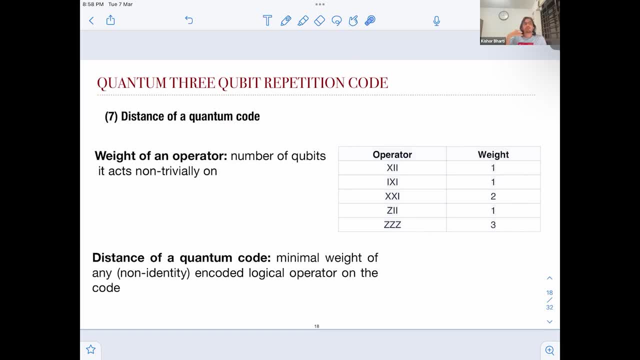 so, finally, you know, like, here we look at the, this motion of distance of a of a quantum code. so here you know, like we have, we define this motion of, you know like weight of an operator. so, similar to the earlier case. in the earlier case we had, you know, the number, the minimum number of bits required. 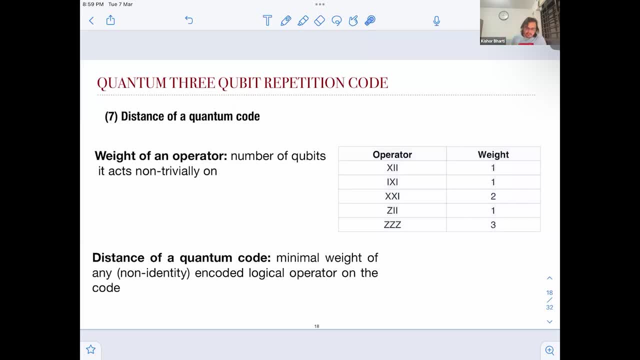 you know like we will use similar idea to define the distance. but yeah, like we will use, we will generalize it And to generalize that, we use this notion of you know like weight of an operator. So so weight of an operator is basically number of qubits. it. 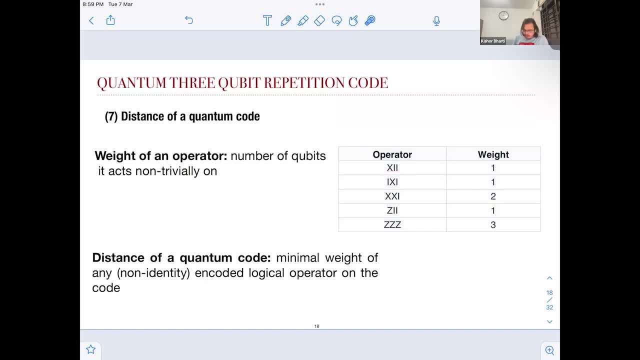 acts non-trivial on. So for example, xii, its weight is one, Zz, its weight is three because it acts non-trivial on three qubits. And similarly xxi, here the weight is two. So the distance of a quantum code like is nothing but minimal weight of any non-identity. 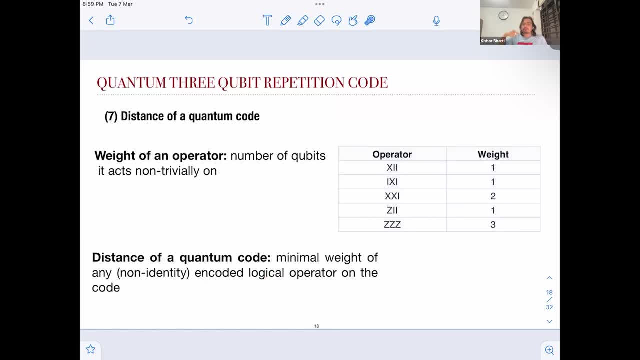 encoded logical operator on the code, because that will take you, you know, like one codeword to another, and we are interested. So basically like, if you think about it, if you so, the so identity is not an error, but on the other hand, if, let's say x or z, error occurs you. 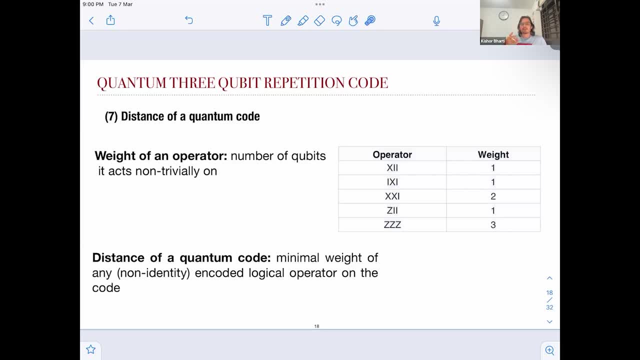 know like that can, like you know, take your like that. that can basically take your state outside the code space. Now, if you had, you know, like, if you have, the number of single qubit errors that occur is. 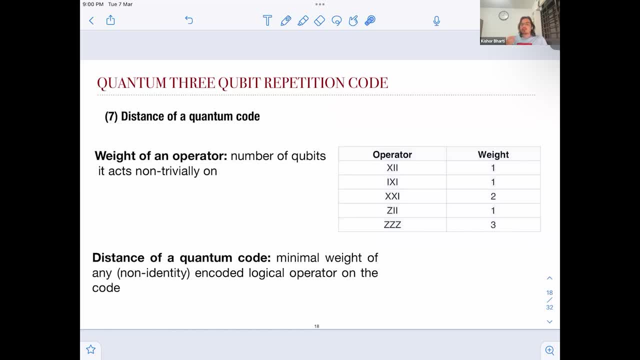 equal to weight of a logical operator, then you will, then your state will remain inside the code space, but you will not be able to detect it. Similar to the case, you know, like the previous case where you had like zero, zero, zero, and let's say, if you have you, 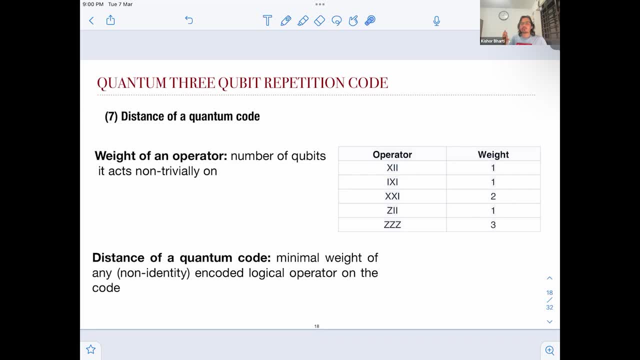 know like errors occurring that all three places, you know like you will not be able to detect it. So so, yeah, I mean. so the motivation is same as the classical case. You basically look at the minimal weight of any non-identity encoded logical operator. 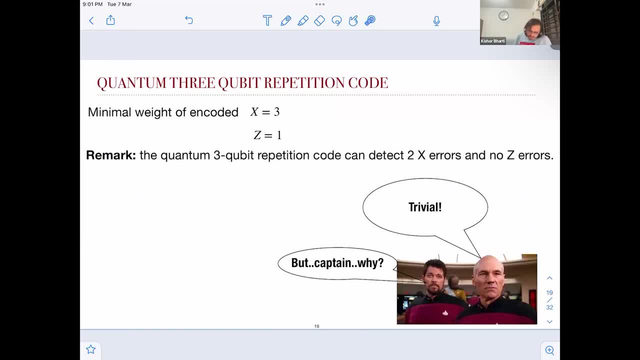 on the code, So so. so so, for the quantum, you know like three qubit repetition code, the minimal weight of encoded x, you know like, yeah, like if you look at, you know, like for the, for the x, like you, 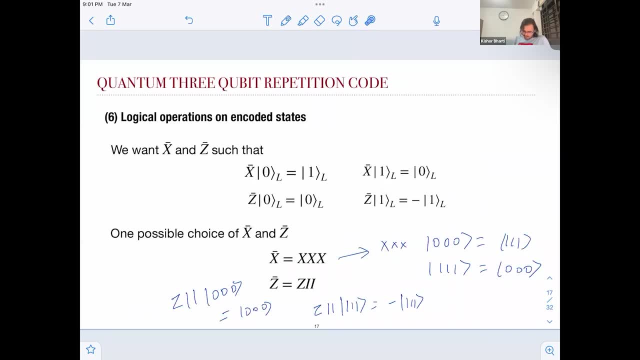 know the minimal weight here is, you know like three, because, like some of you are, I think, yeah, like I'm seeing in the comments, you're writing like why not I z z, why you not z z, z? like I mean, there are many possibilities, but I'm saying but for x. 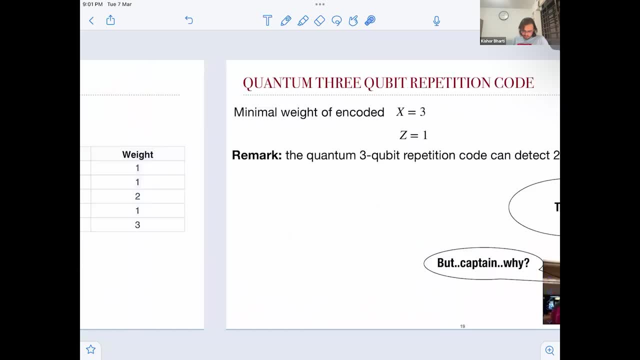 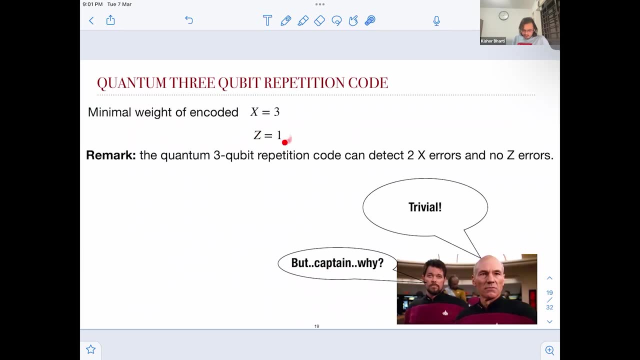 there is just one possibility, like x, y, just x, x, x. like you know, just one possibility. but on the other hand, for the z, if you look at the minimal weight of the encoded z, you know, like it's it's, this is one. So the quantum three qubit repetition code can detect. 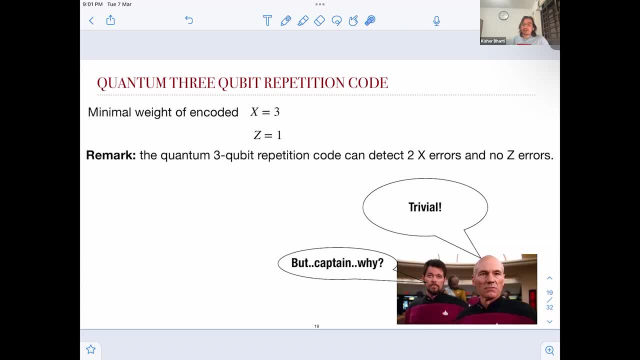 two x errors and no z errors, And why that is the case. I mean you can see it, because you know like if, let's say, one z error occur, it can take you, you know like it can keep. 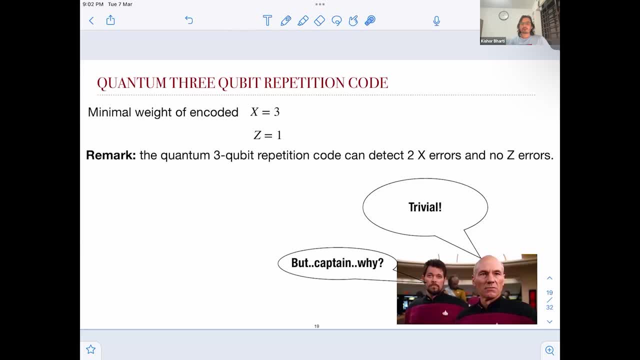 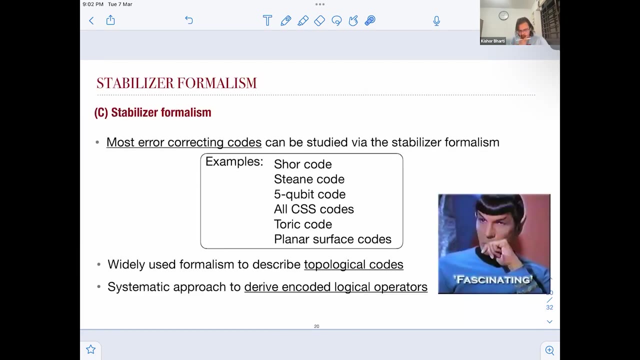 you inside the code space and you know like you will not be able to detect it. Nice So, and it makes sense, because you know this quantum three qubit repetition code is pretty much a classical. Nice So to understand all this, like in a more systematic fashion. 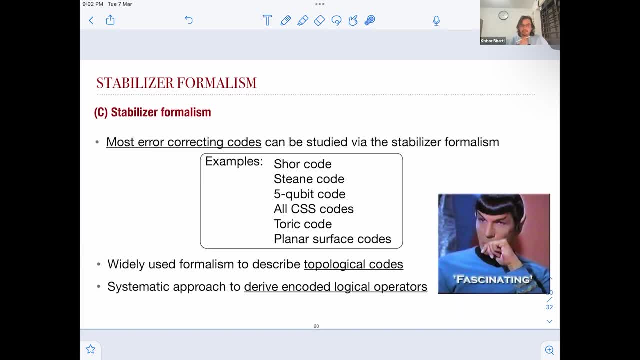 you could use something called a stabilizer formalism And, and actually most error correcting codes can be studied via the stabilizer formalism. So so the idea is simple, you know, like I mean, I will explain later. And they're, like you know, codes, like you know, short. 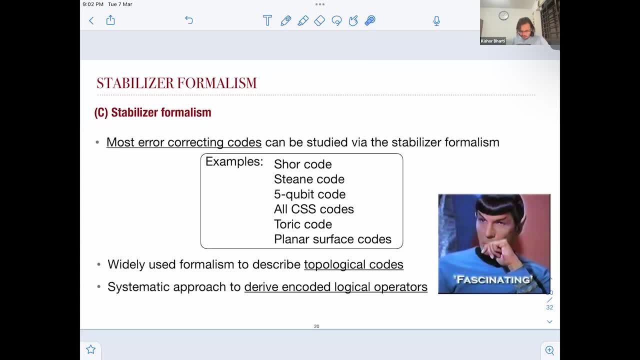 code, string code, five qubit code, like CSS codes, Tori code, like planar surface code, like like this can be studied, you know, like using this stabilizer formalism, And this is formalism that is widely used to describe topological code. So later, when I will talk, 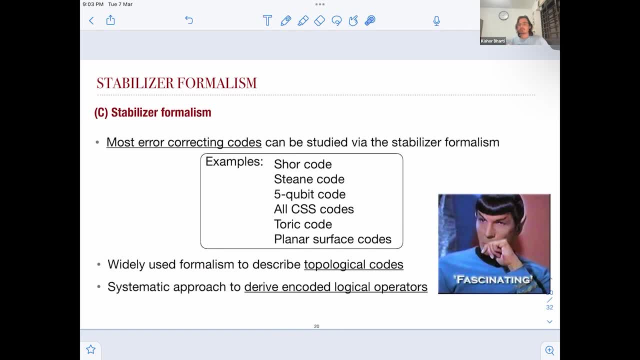 about topology in one of the tutorials and topological code. you will see that you know like it's very much related to stabilizer formalism And it's a systematic approach to derive encoded logical operators. So you will see that the logical operator that we 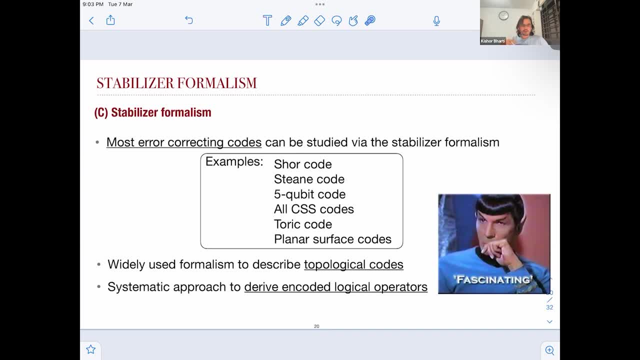 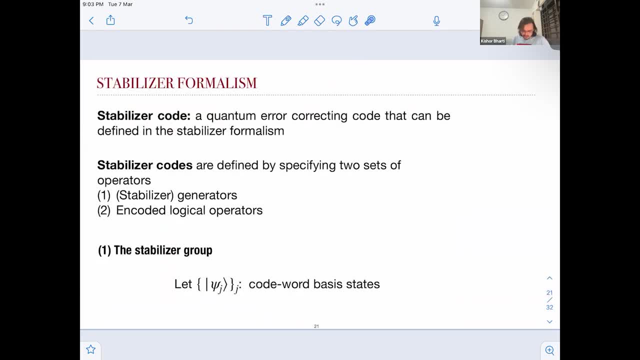 fashion. So a stabilizer code- you know, basically it's a topological definition- is a quantum error correcting code that can be defined in the stabilizer formalism. And so, basically, to define a stabilizer codes, you need to specify two sets of operator. 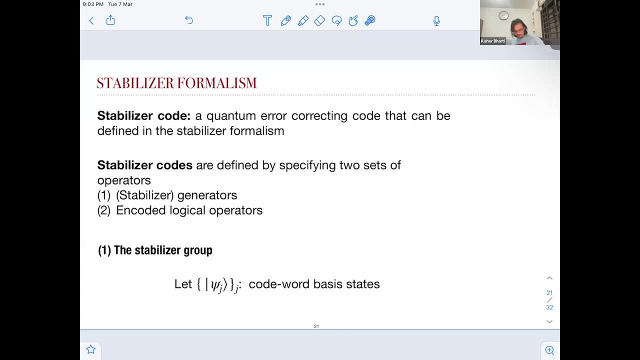 something called a stabilizer generators and the encoded logical operators. So we will see, you know, like, what they are. So let's you know, look at the stabilizer group first, because we are talking about stabilizer generator. So let's say you know, like with the set of code, word, basis of states. 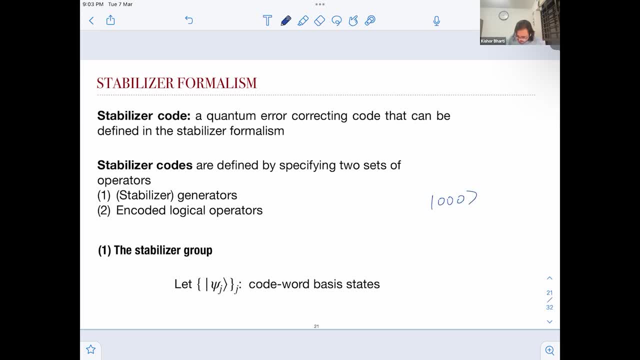 So, like for example in the previous case, you know like we had 0, 0, 0, and 1, 1, 1, these were the code word basis states. So let's say, you know like in general, 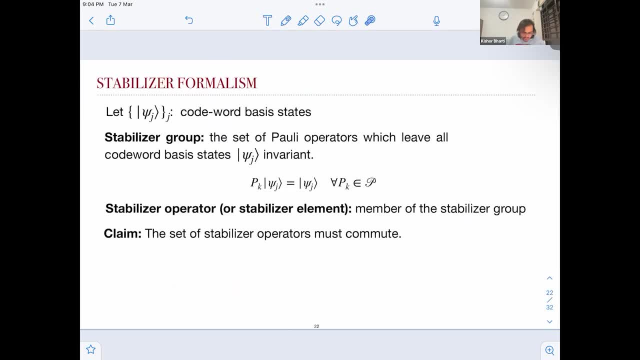 you have, you know this size, this set of code word basis state, And the stabilizer group is basically the set of poly operators which leave all code word basis states. you know like invariant. So basically you know like let's say PK. you know like. 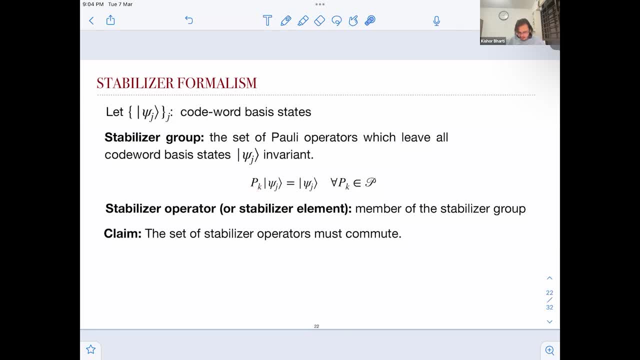 so all those poly operators which act on size, you know, like, you know, I think this should be some yes or no. So basically, all those poly operators which belong to a particular set and which you know like, leave your code word basis states invariant. they will be. the set will define. 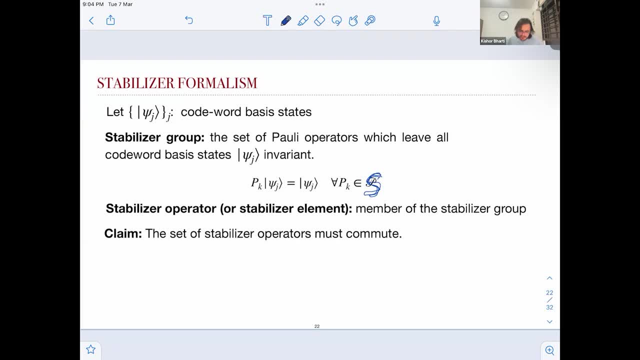 a group called the stabilizer group and the stabilizer operator or stabilizer element that will be a member of the stabilizer group. so the the simple claim that you know the setup of stabilizer operators must commute when uh, like you can, in fact you know like uh show contradiction that 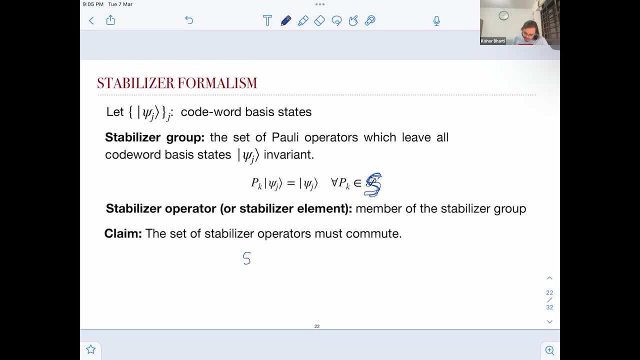 you know like, if they don't commute. so let's say you have two stabilizers, let's say s, s1 and s2, and let's say, if they're, if they don't commute, uh, then because we know that you know like, since their fall is, you know like, uh, so we will be interested in poly stabilizers, so they. 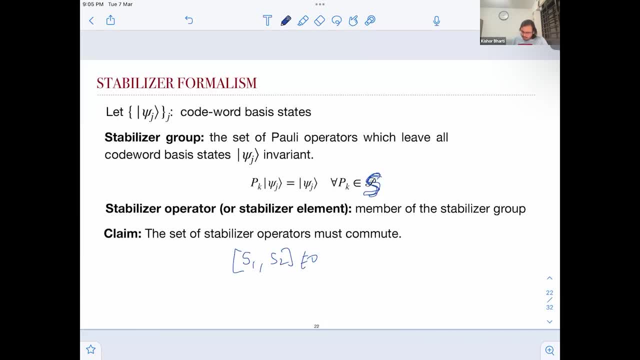 are they either commute or they, or they anti-commute. so let's say, if they don't commute, then we have s1, s2 equal to minus s2, s1. and let's say here some state psi, which belongs to the, let's say, size, which belongs to the code space. if you act on s1, s2, you know like uh size that will be. 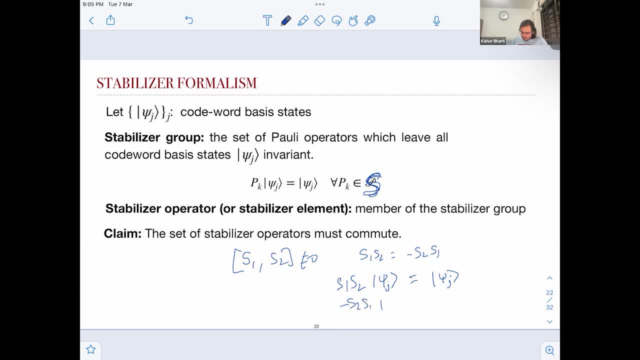 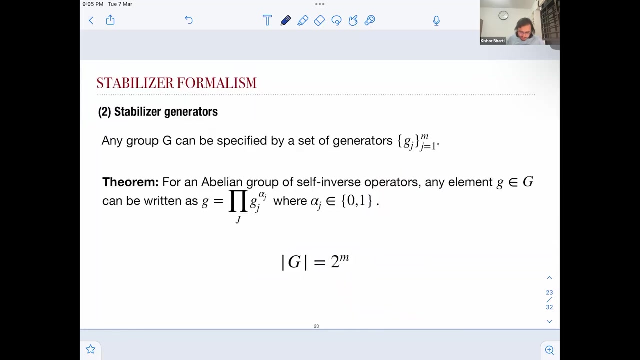 nothing but sizes. but if you act on minus s2s, s1 on size a, that will be minus size. so you have this contradiction and uh, and because of that you can see that, uh, yeah, like they should, uh, yeah like commute nice, very good. so so we talked about even the stabilizer group. 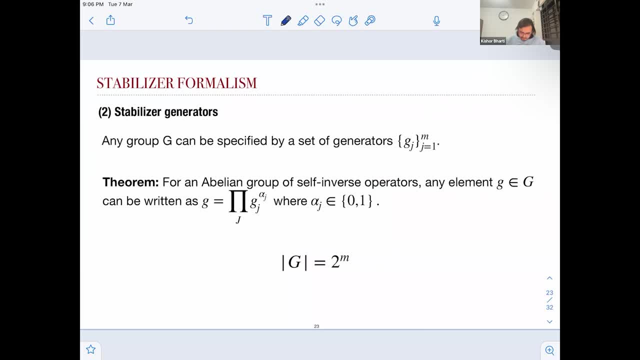 now for a group, you know, like, i mean and uh. you can define: uh, yeah, like, uh, yeah, like, yeah. so so for any group g, you know, interested in all this. so we know that the stabilizer group, there is the element, the, the stabilizer elements, basically they commute, so it's a avilion group like and uh. 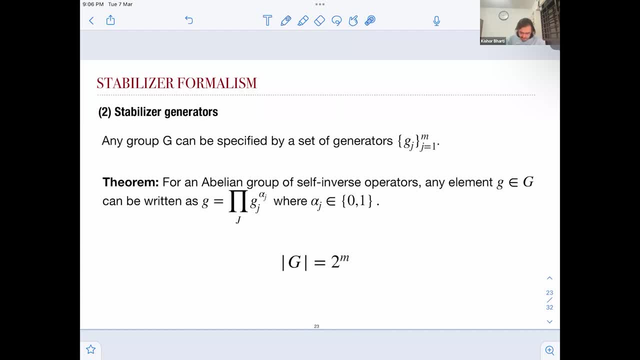 and uh. we know that any group g can be, you know, like a pipe by a set of generators. like you know this gj and uh, this theorem, you know it's the�앣tømü which you can find in, like you know, regular, like you know, abstract algebra textbook that, if you 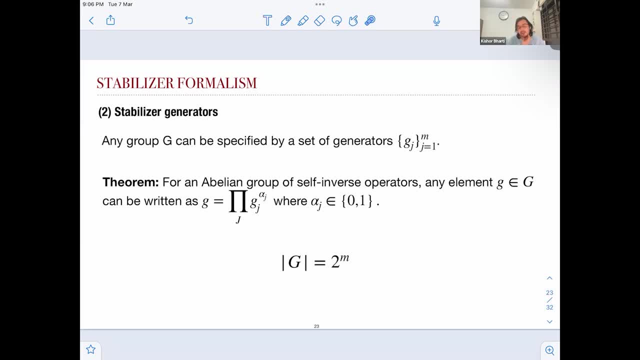 have a avalien group of self-inverse operator- example: you know, like, uh, like polys are one such example, uh, and like you know, and polystabilizers are one such example, then any element g can be written, as you know, like, whatever this formula and you can, you know, like, you show that uh. 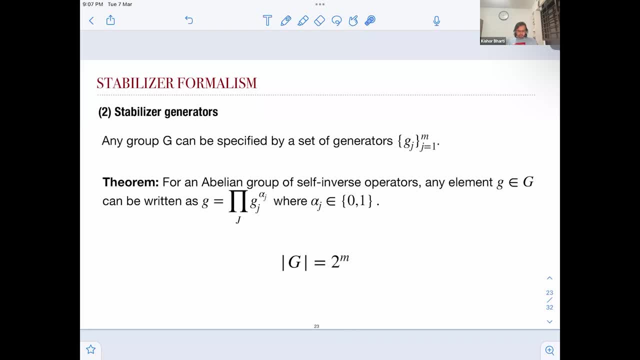 like using theorem that the order of, uh, the group g is nothing, but you know, like two to the power m, where m is number of generators. so one can use this uh, you know, like i notion to basically come up with a simple formula. so let's say you have number of physical qubit, that you have is k. 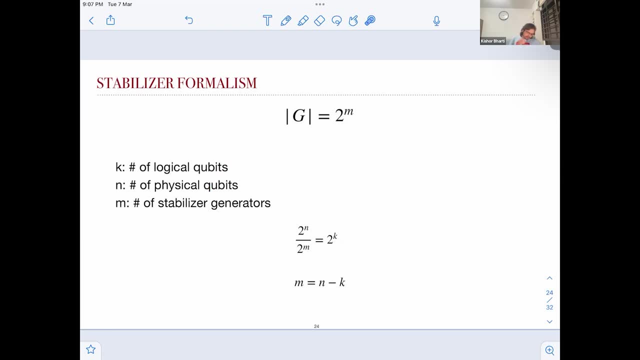 the number of physical qubit that you have is n and let's say m is the number of stable identifiers generators. then basically we know that you know, like the order of this group g is two to the power, n, and so that's, you know, like the, the, yeah, the, that's basically your, your uh codes, like you know. 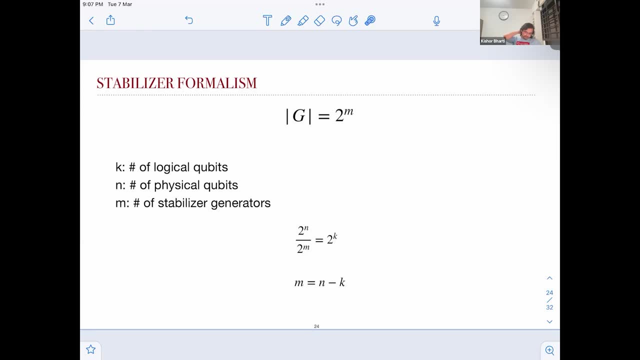 i mean, yeah so. so basically every stabilizer you know like is dividing your hilbert space in two part, depending on whether you get the plus one eigenvalue or you get minus one eigenvalue. and the size of the entire hilbert space is, you know, like two to the power, n and uh, and you are basically dividing it. you know like uh m times. so 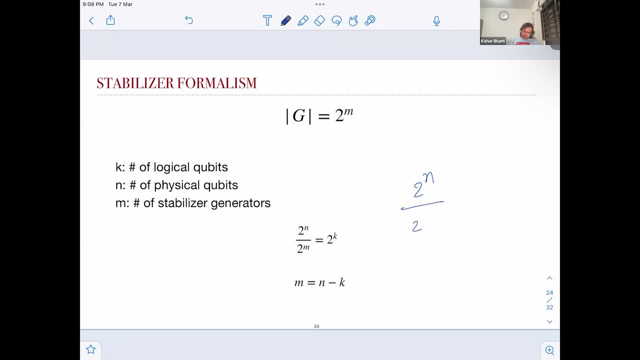 you know like so, and every time you divide it by half you have, you know like, two to the power, m times you know like, uh, that will be, you know like, the final size of the of the hilbert space, which you know like, which will you, which you will use as a code space, so that will be known at two to power. 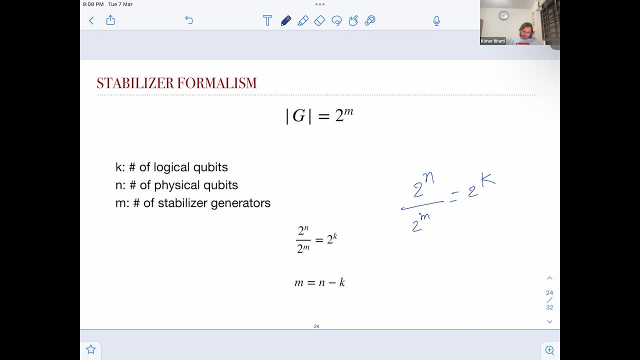 k and then by taking log, you can you know like you can instead like see that this n is nothing but m plus k, and then from where you will get m equal to m minus k. so this simple relation is still. so i mean for them. but let's say, even if it's become abstract, you can just see that you know. 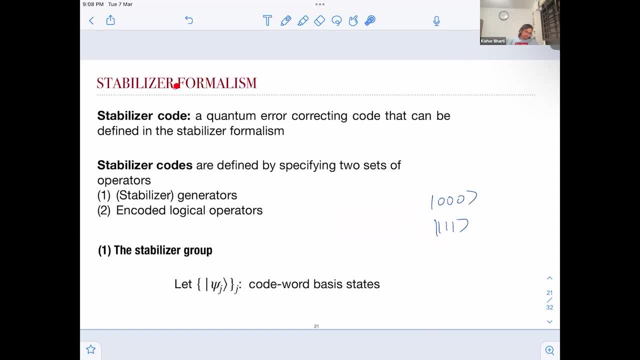 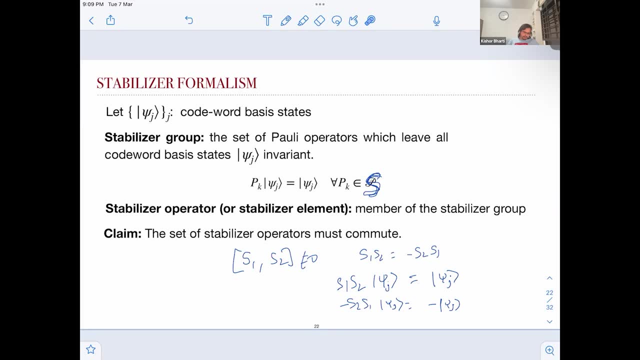 like we are talking about. you know like, uh, like this formalism called stabilizer formalism, where we have a set of poly operators which you know like, which commute and they leave, you know like a set of poly operators which you know like, which commute and they leave, you know, like a set of poly operators. 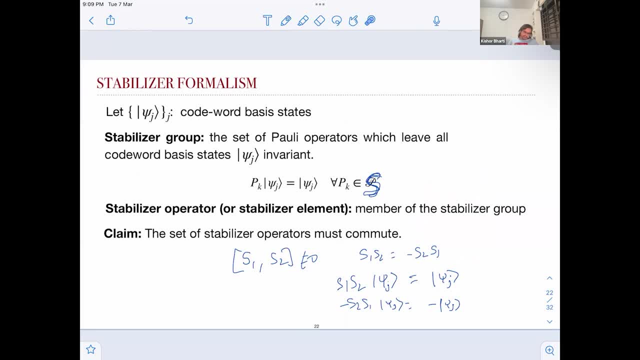 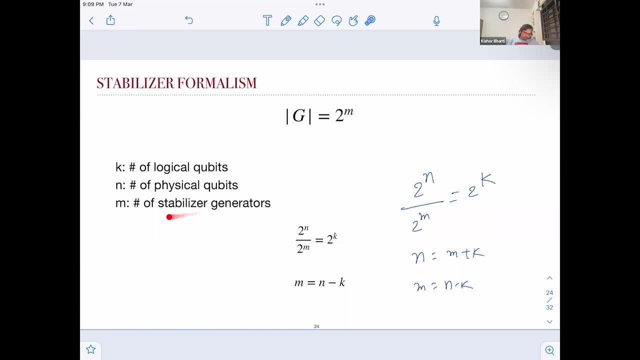 subspace, basically in a variant, and uh, the elements of this, you know, like this group, basically they are called stabilizer, like a stabilizer operator or stabilizer elements, and then, uh, i just you know, like i just uh showed that, uh, basically the number of stabilizer. 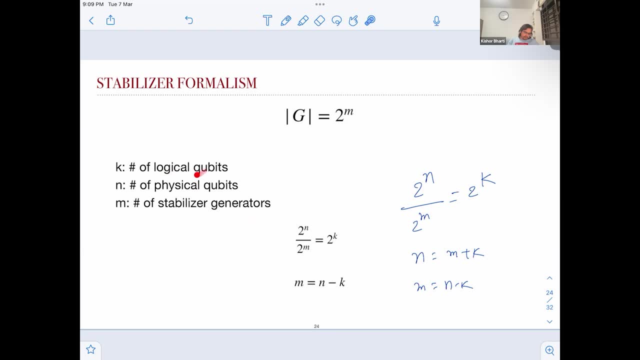 generator that you have. it's related to number of physical qubit and number of logical qubits. so you can see that by if you increase your number of stabilizer generators too much, your number of logical qubit, may you know like, may decrease. yeah, so let's look at, you know, like the 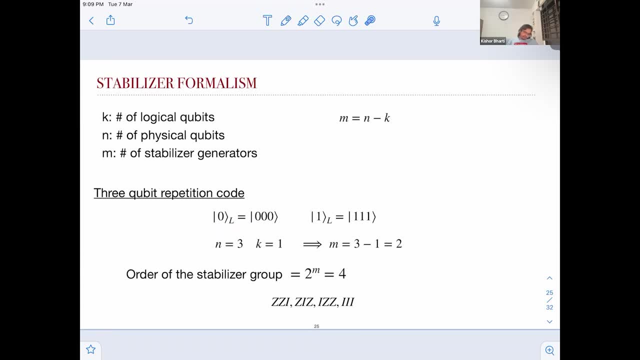 three qubit repetition code. so for the three qubit repetition code the zero logical is zero, zero, zero. one logical is one, one one, so the n is here three, k is one, so m is basically three minus one equal to two. so you have two stabilizers here and the order of the stabilizer group is basically two. 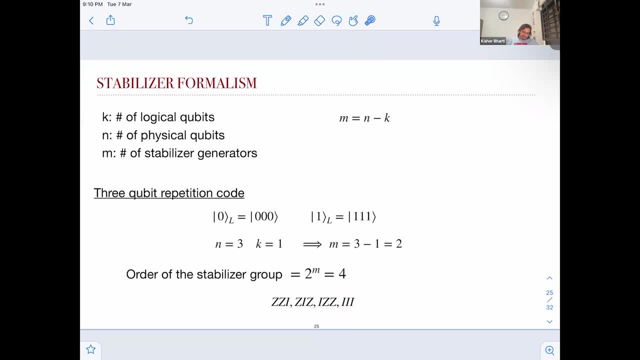 to the power two, that is four, and you can see that there are these four stabilizers which can, which stabilize, you know, like zero, zero, zero, and one, one, one, like i mean any element in the subspace, yeah so, uh. so, basically, if you say, if you act on jzi, or let's say, zero, zero, zero, you. 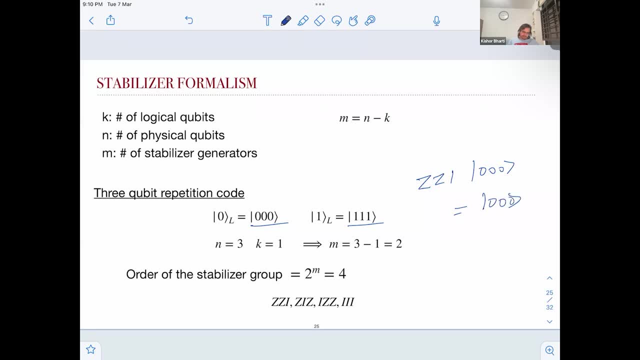 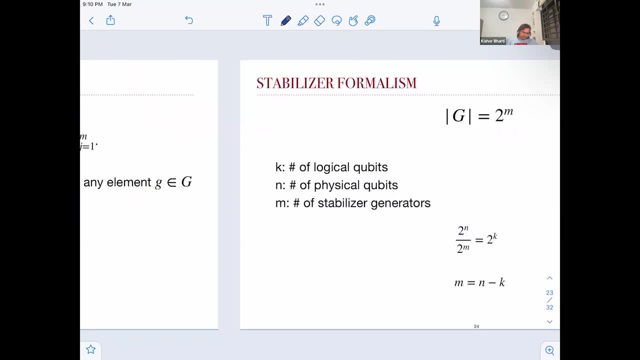 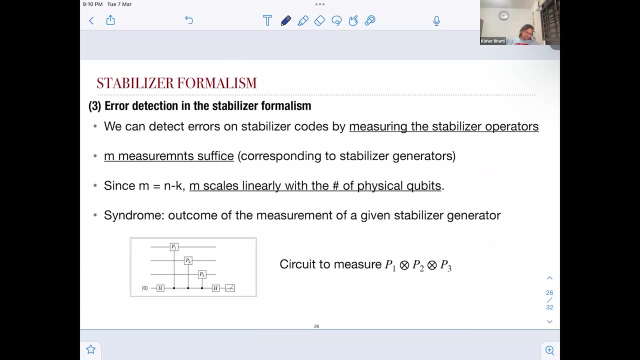 know like you get again zero, zero, zero. yeah, got it so. so we talked about you know like uh, uh, so far, yeah, like a stabilizer group and a stabilizer generators. another question becomes: how can you use this formalism to detect error, so we can detect errors on a stabilizer code? 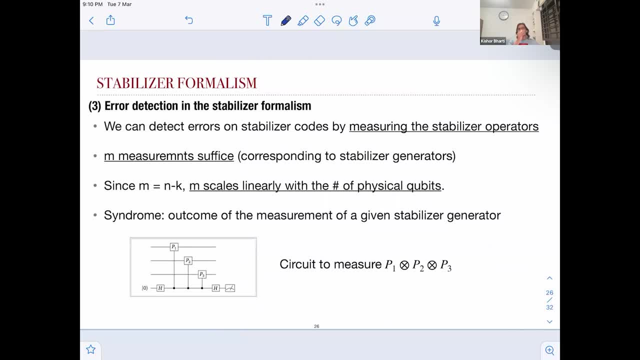 by measuring the stabilizer operator. so let's say, if your, if your core, if your state is in the code space, then it should be stabilized by the stabilizer operator, which means you know like it should correspond to plus one eigenvalue. on the other hand, if you measure it and you get. 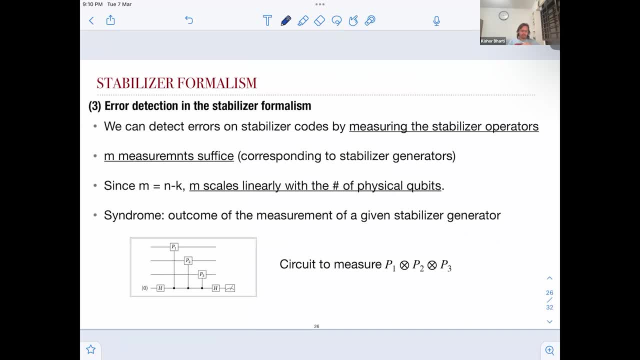 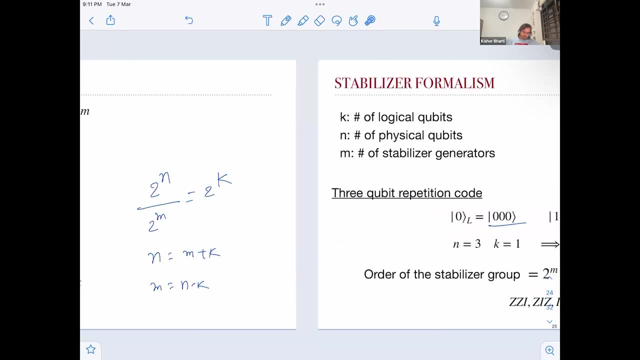 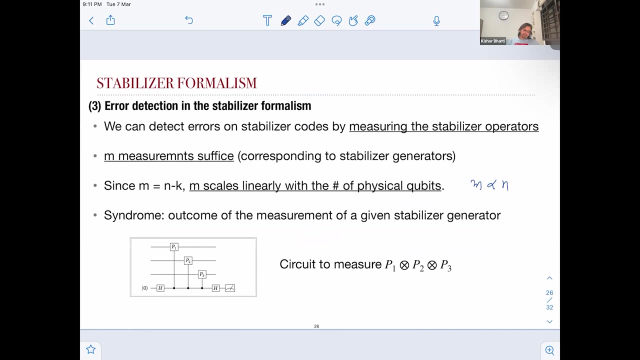 minus one eigenvalue, you will find that something bad has happened. and in fact, you know like you can just measure the stabilizer operators and m measurements will suffice, like you know, and that, should you know like follow from the previous revelation which i mentioned here. and since m is n minus k, you see that your m basically scales linearly with m. so so the 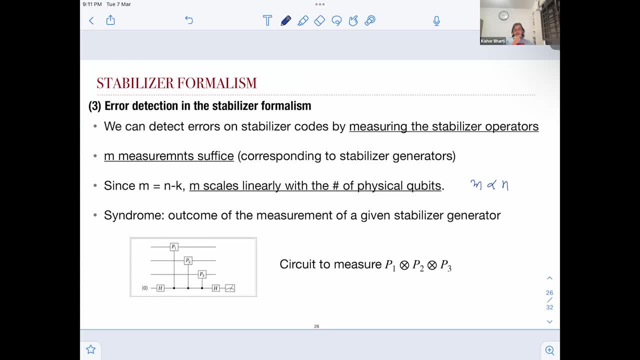 number of measurements that you need to perform. like an m, uh, it scales linearly with the number, which is good, and normally, like you know, in the, in the, in the quantum error correction lingua, people talk something like syndrome, which is, you know, like outcome of the measurement of a given stabilizer generator. so so you have, like you know, m. 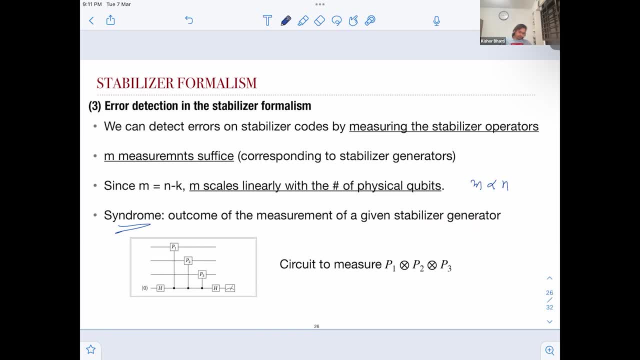 stabilizer generator and, corresponding to that, you know like you will have a bunch of one one, one minus one, one minus one, something like you know, um, and these are basically your, your syndromes, and by looking at your syndromes you will find out, uh, whether an error has occurred or not. so 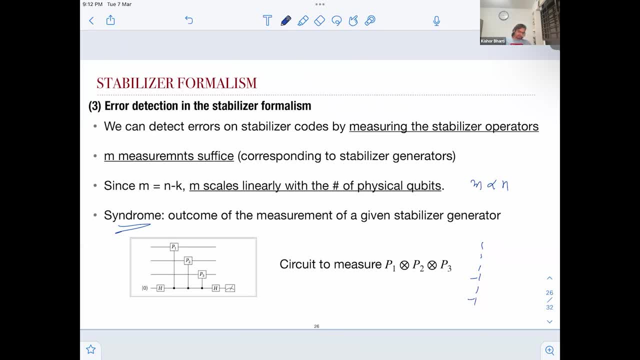 for example, this is a circuit which can be used to measure, you know, like p1 tensor, p2 tensor, p3, where you know like pi or some for that price. so we talked about, you know, like how can we detect the error? so, to detect error, it's, it's uh, it's simple. you basically just uh, yeah, like you measure. 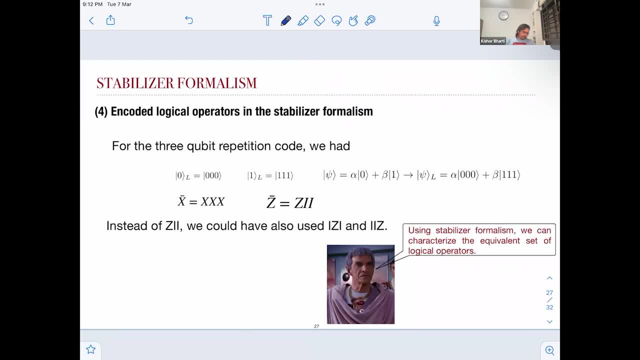 your stabilizer operators, uh, now the logical operators. you know like that's also very uh like easy to see in this framework. so, for three qubit repetition code, you know like we had, like you know, zero logical zero, zero, one, one, logical one, one one, and this was our, you know like, state in the code space. the x bar that we chose was x, x, x. 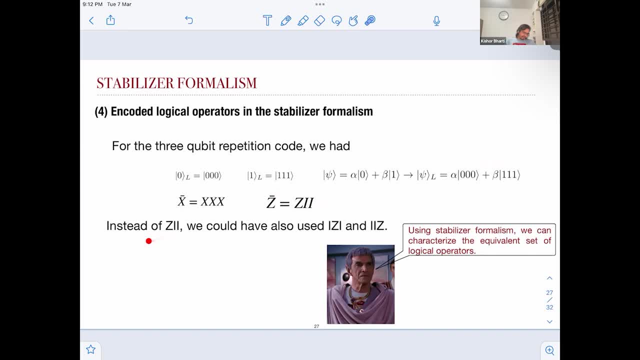 and z bar. was z i now instead of z i i. we could have also used i z i and i i z, or you know like, or let's say zzz and like you know. you could have used any of this now, so you can see that there's. 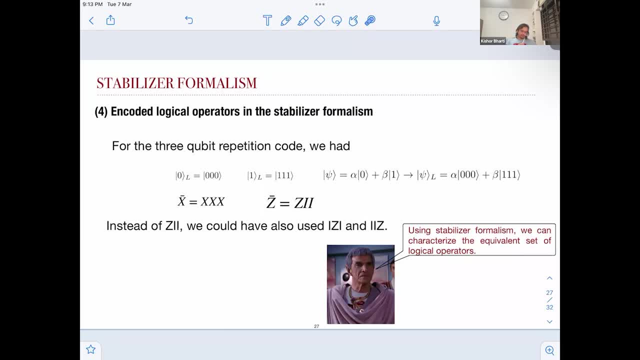 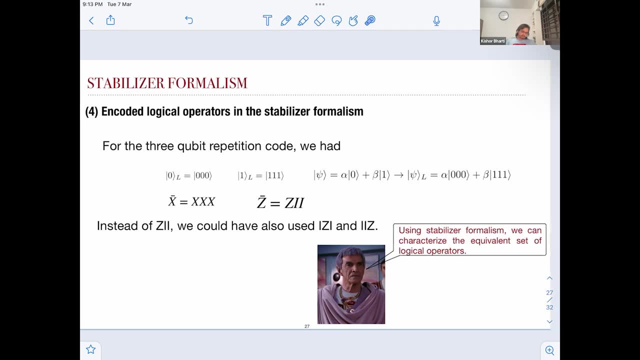 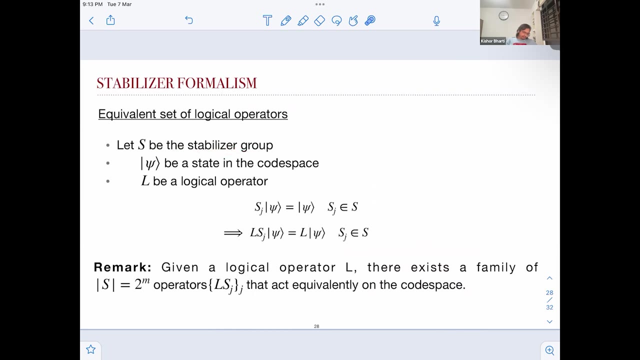 the equivalence of logical operators that you could have used and actually, using the stabilizer formula, you can characterize this equivalent set of logical operators. so let's look at what are these equivalent set of logical operators? so let s be the stabilizer group. let psi be a you know, like state in the pole. 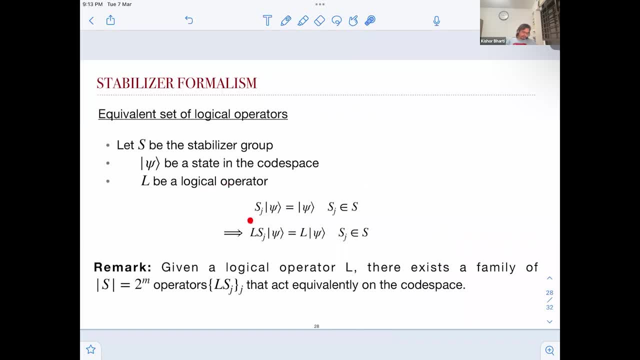 space, l be a logical operator, then we for any sj which you know like, which is, which is in the stabilizer group, sg acting on psi, will be psi. now if you act on your sj, psi by l, that will be also l sine. so you see that if f for l being a logical operator, lsj is also a logical operator. so, given a, 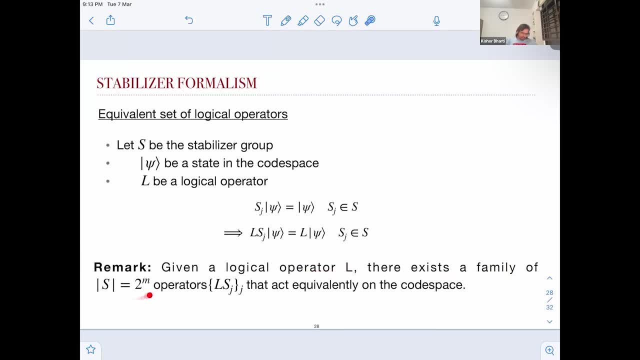 logical operator l. there exists a family of you know, like two to the power l operator, lsj, that can that act equivalently on the code space? so basically the action of a logical operator operator is up to a stabilizer. because you can add a stabilizer and it will, it's like 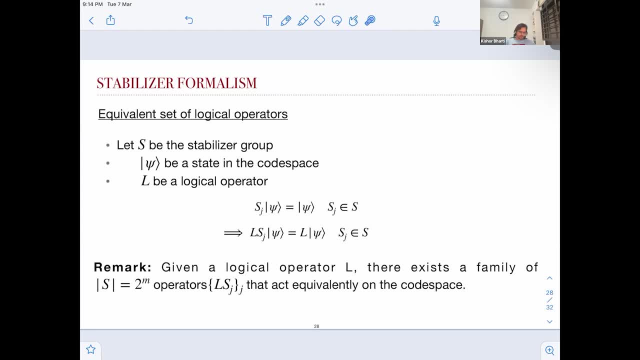 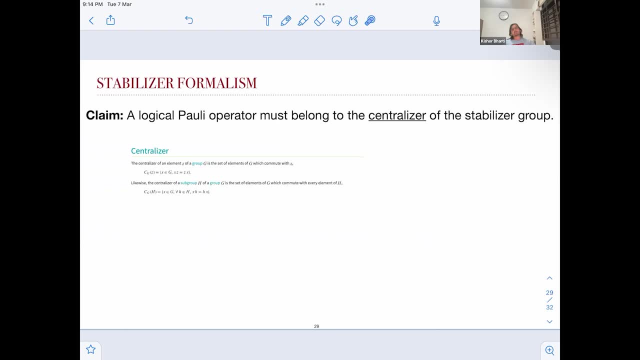 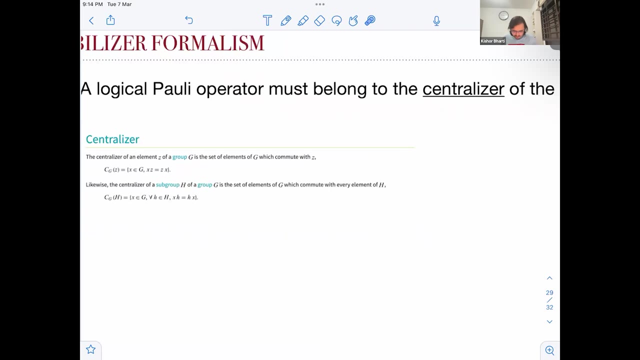 you know, it's like nothing happened. yeah, yes, so a logical operator basically must belong to. you know, like, the claim is that a logical operator must belong to the centralizer, the stabilizer group, and and this you can see, you know, like, uh, like. so the question so, basically, 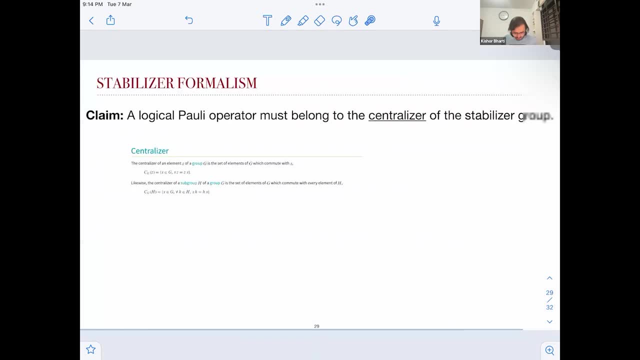 how do we find, you know, like, what are the? you know the, you know the, the logical operator. so, basically, to do that, you need to just, you know, like, look at, so you have a stabilizer group and you need to find the centralizer, and and then the question becomes: what is? 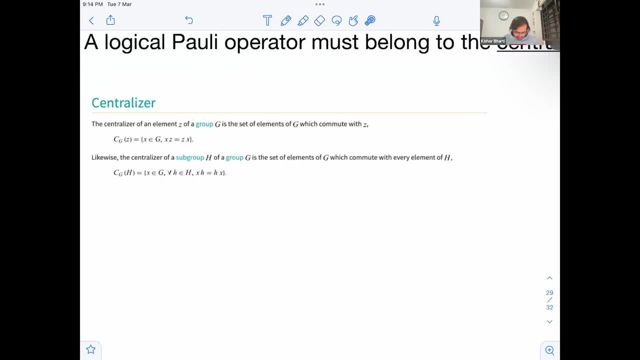 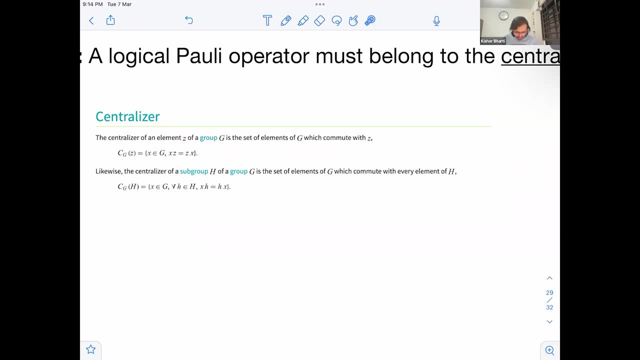 a centralizer. so you can see, you know, like, from the ball frame i have taken this definition. so the centralizer of an element z of a group g is a set of element which commutes, which, so you know like, all the elements which you know like, which basically commuted between: 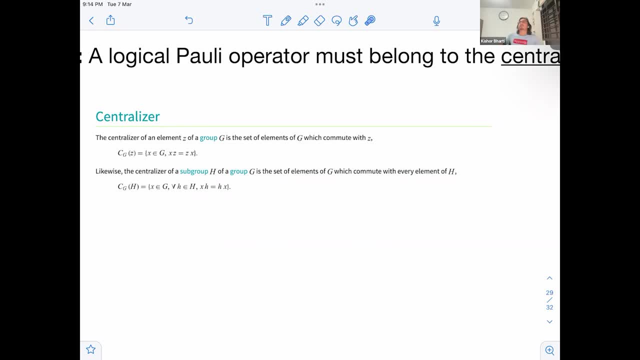 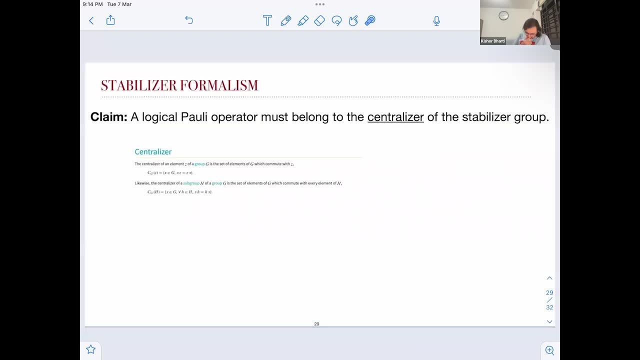 you and uh, yeah, so you see that, uh, why it should happen, like you know. uh, uh, yeah, like so, basically, yeah so. so the logic operator, i mean it, must commute with every element in the stabilizer. if it does not commute, so let's say no, it does not belong in the stabilizer, in the centralizer. 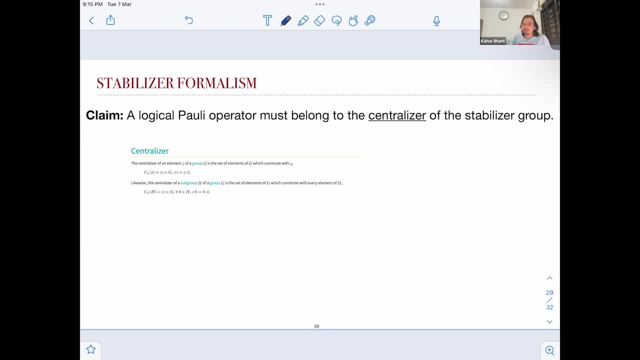 then you know like basically it will not commute with- uh, you know the elements in the stabilizer group and if it does not commute, then you can again show the contradiction that, uh yeah. so for example, let's say l, and you know like does not commit with some stabilizer sj. so 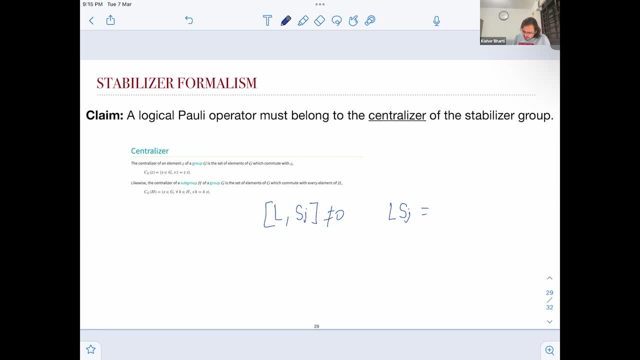 lsg, let's say non-zero. so then we have, you know like, lsj is equal to minus sj, l, because we are are interested in poly operator. Now, if you act on L S j, on some let us say some quantum state psi, which is in the code space, you get L psi. Let us call that. you know like. 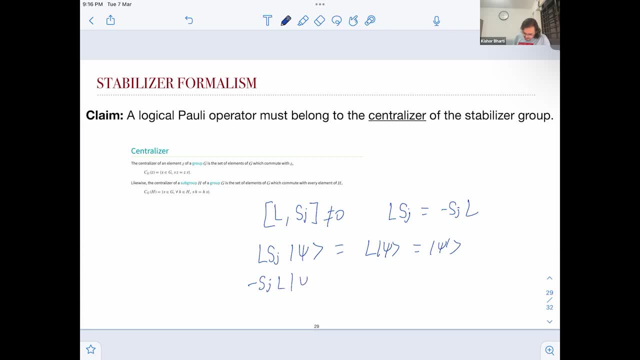 psi prime. On the other hand, if we take minus S j L and act on psi, that is minus S j, acting on psi prime, that is minus psi prime. So again you see a contradiction. So basically, you have, you know, like your logical poly operator, They, basically, they must belong to the centralizer. 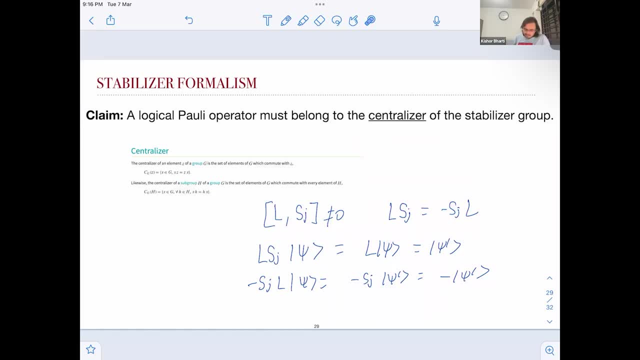 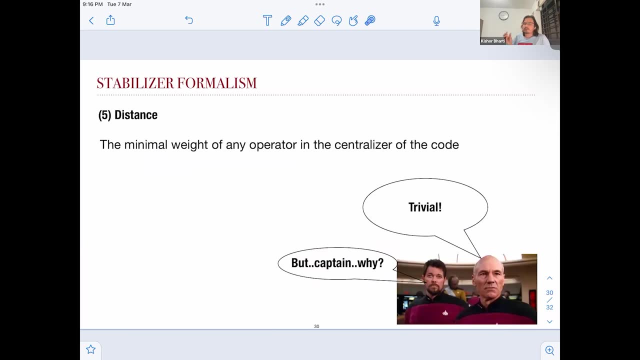 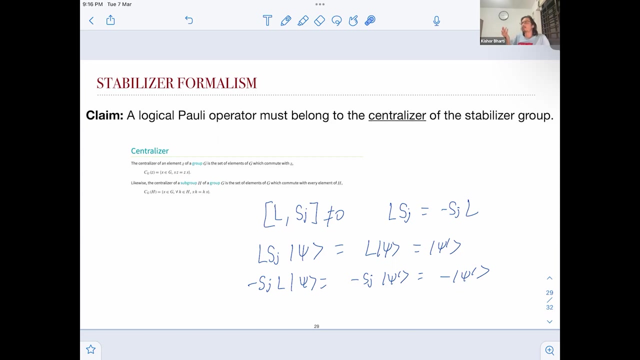 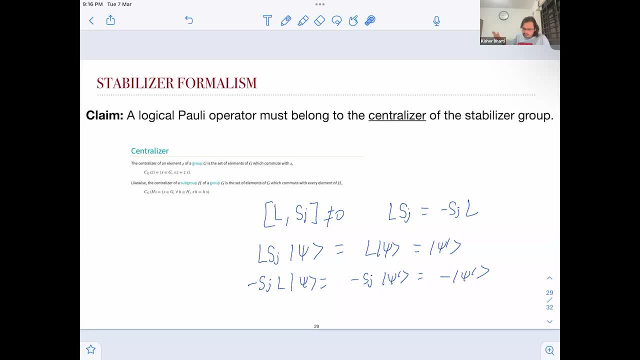 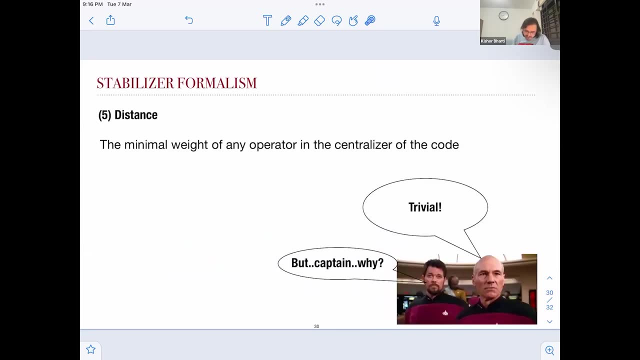 the generator and that will give you, you know, like the stabilizer group, and from there you can get the state of the centralizer and the distance basically is nothing, but you know the minimal weight of any operator in the centralizer of the code and why that should. 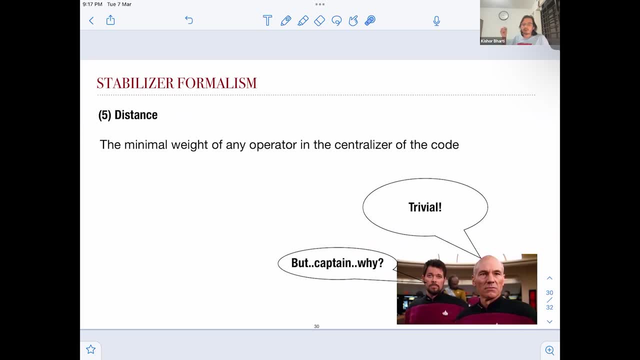 happen because, you know, like the logical operators, they belong in the centralizer of the code and the definition of distance is basically a minimum weight operator. like you know, minimum weight logical operator and since the logical operator belong in the centralizer of the code, the minimum weight operator in the centralizer of the code will give you the distance of the code. 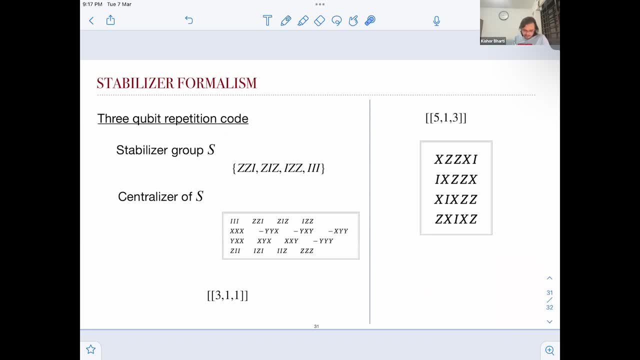 Okay, So let's look at: you know like the three qubit repetition code. So you hear the stabilizer groups are basically, you know ZZI, ZIZ, IZZ, whatever generally Centralizer you can you know like calculate, these are the ones and you can see here that you know like the minimum weight polyopator is one, so you know.